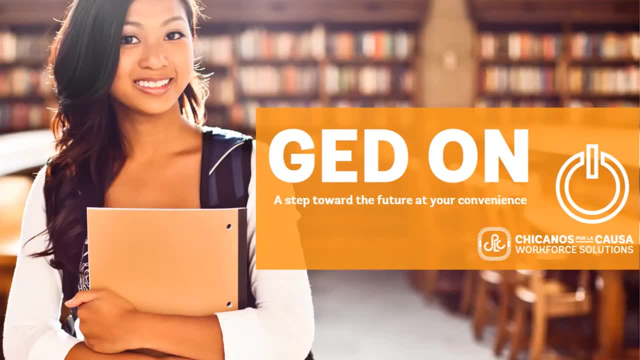 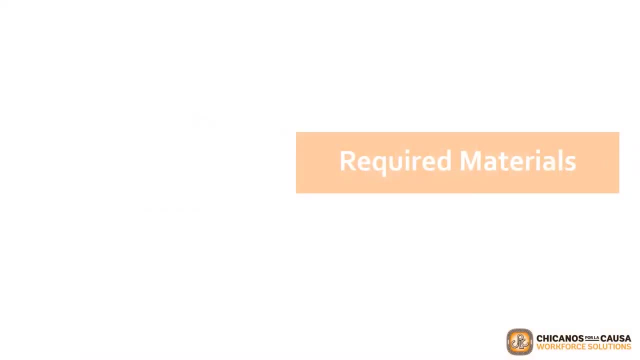 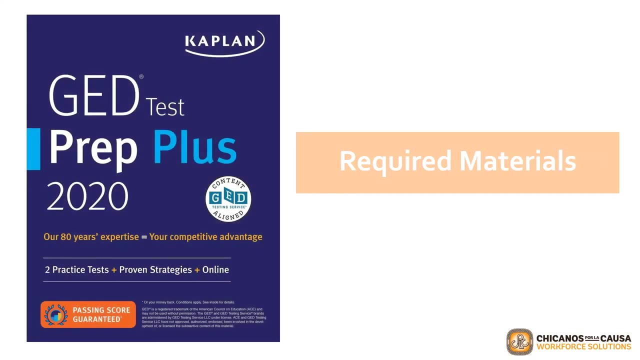 keep up. As a reminder, we'll be using the Kaplan GED Test Prep Plus 2020 book for Chapter 1 and all chapters of the chapter. The book is covered within the GDOn platform. You can find links below to purchase the book. 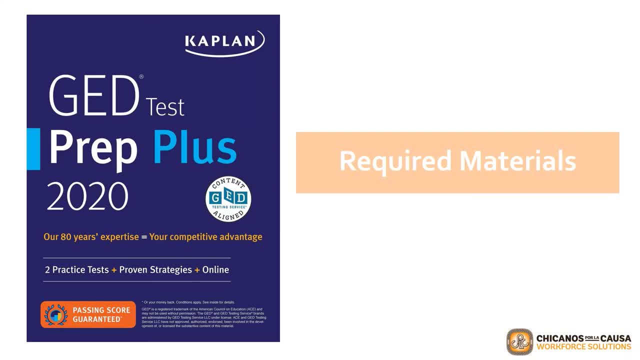 at local stores or online. Also, please remember that your book contains access to the Kaplan Online Center, which contains access to additional instruction and practice materials that will assist you in being successful on the big test day. Now, before we start on Chapter 1,, I want to cover some information regarding the math. 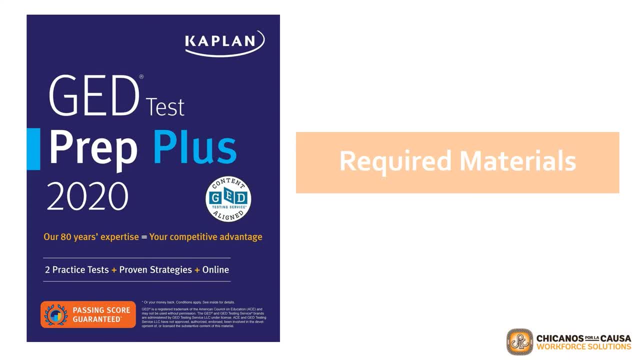 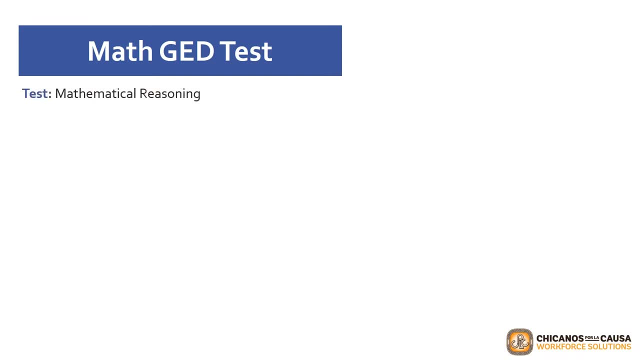 test on the GED. The Math GED Test. Prep Plus 2020 is an educational video that will help you learn more about the GED. The Math GED Test. The test itself is called Mathematical Reasoning Time-wise the test. 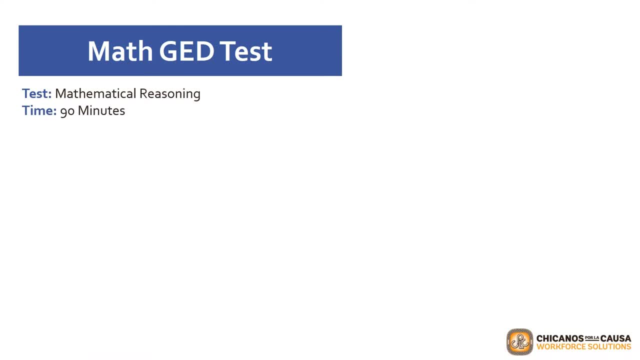 lasts about 90 minutes. Now, within these 90 minutes, you'll be answering approximately 46 questions that will vary in type and form. Now, these questions are going to be offered in the format of either multiple choice- fill in the blank, drop down, drag and drop- or 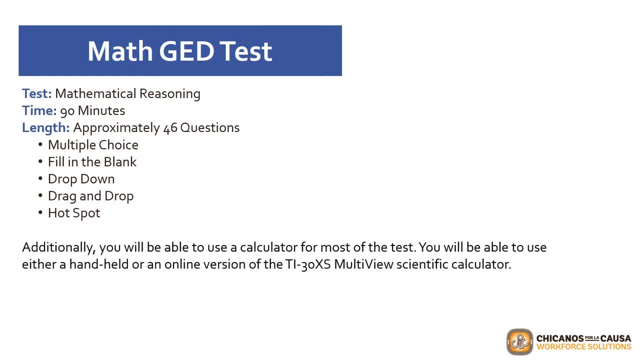 click on any of them. Additionally, you'll be able to use a calculator for most of the test. You'll be able to use either a handheld or an online version of the TI-30XS MultiView Scientific Calculator. Please be aware that you will not be able to use a calculator for the first five questions. 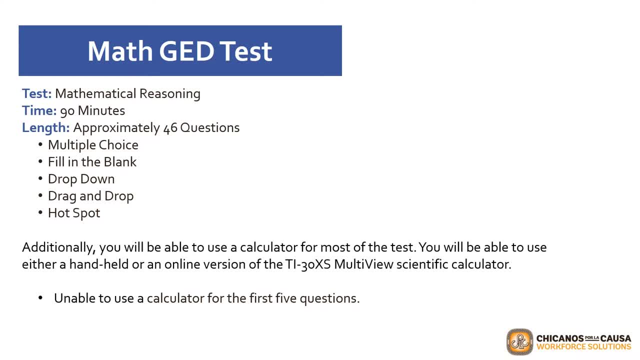 on the test. It is highly recommended that you take your GED math test immediately after completing this section of the book. That way, all of the information that you've learned and gained is fresh in your mind and, ultimately, will lead you to have a successful test result. 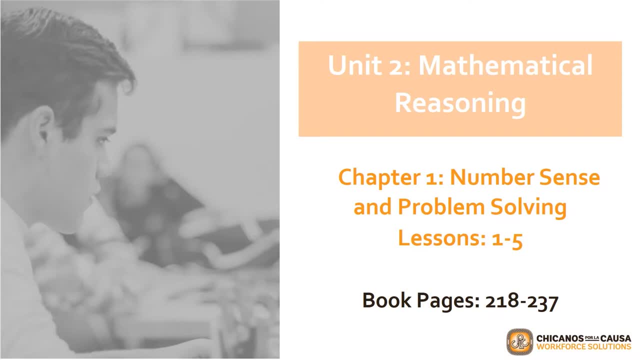 We'll be starting our first video by covering Unit 2, Mathematical Reasoning- Chapter 1, Number Sense and Problem Solving. Chapter 1 will be covering lessons 1 through 5, starting on page 218 of the Kaplan book. So let's go ahead and begin. 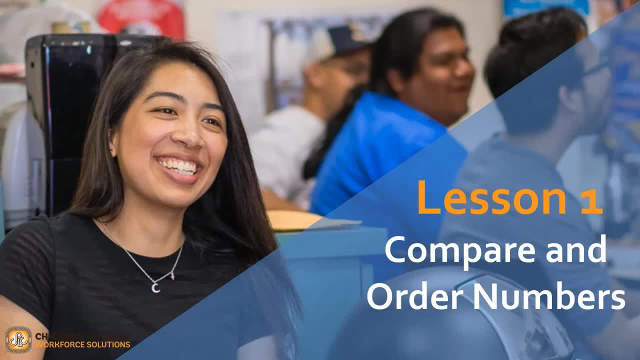 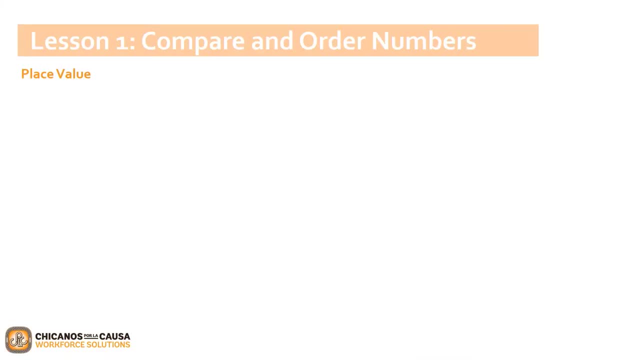 Let's begin with Lesson 1,: Compare and Order of Numbers. Numbers are part of the everyday life. This can be with paying with cash, reading a bus schedule or changing a television channel. You're using whole numbers. The value of a number depends on the place value or its digits. 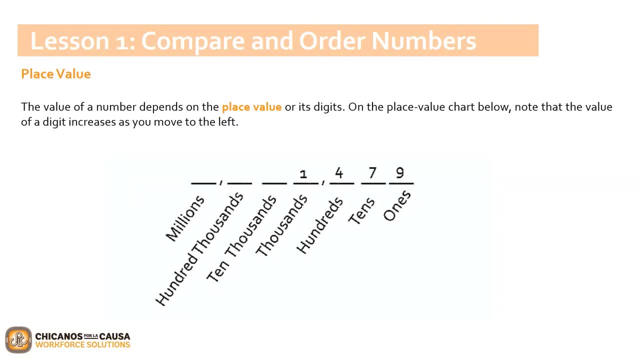 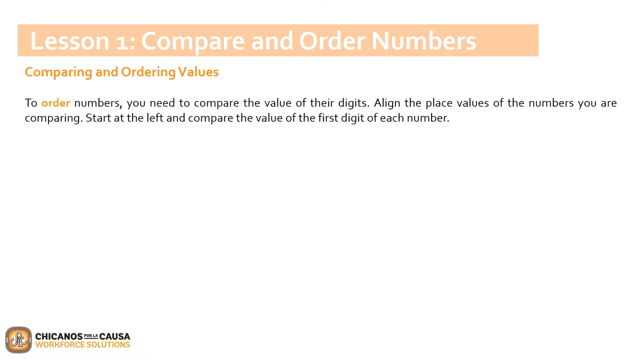 On the place value chart below. know that the value of a digit increases as you move to the left And the whole number shown on the chart 1 has the greatest value. The number would be read as 1,479.. To order numbers, you need to compare the value of their digits. 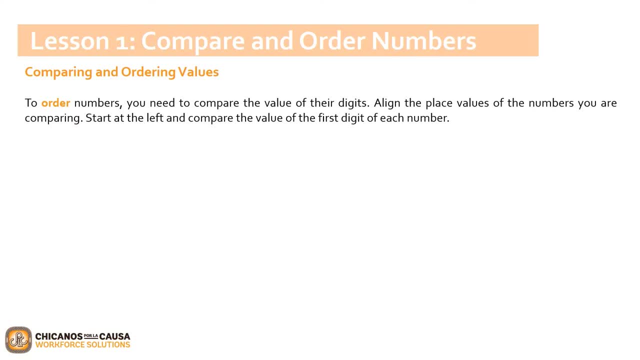 Align the place values of the numbers you're comparing. Start at the left and compare the value of the first digit of each number. For example, place the numbers 352,, 95, and 310 in order from least to greatest First. compare the first digit of each number. 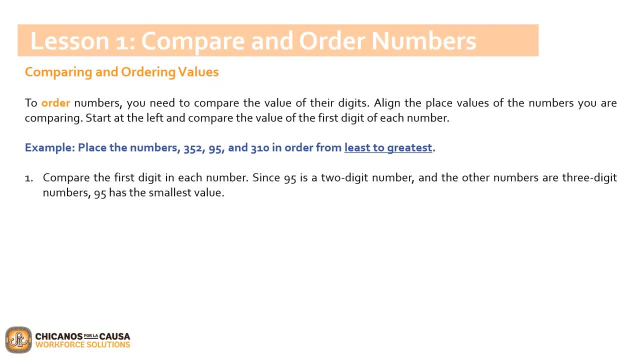 Since 95 is a two-digit number and the other numbers are three-digit numbers, 95 has the smallest value. Next compare the first digit of the remaining numbers. Since both numbers have the same digit, 3, in the hundreds place, compare the digits. 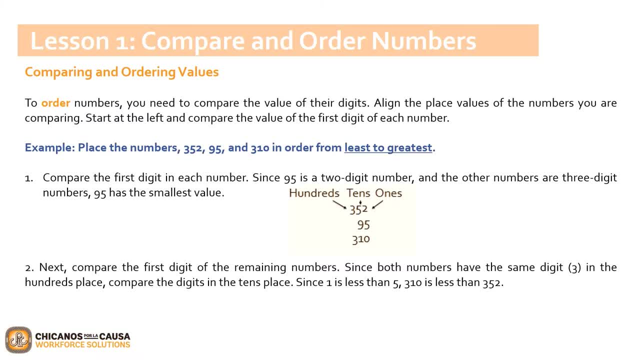 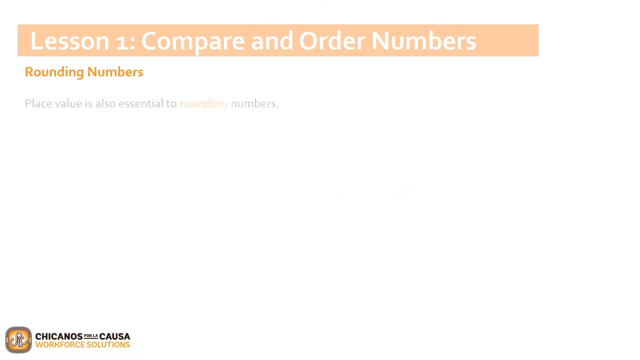 in the tens place, Since 1 is less than 5,, 310 is less than 352.. Therefore, from least to greatest, the following numbers would be placed as 95,, 95, 95, and 310,, 95,, 95, and 352.. 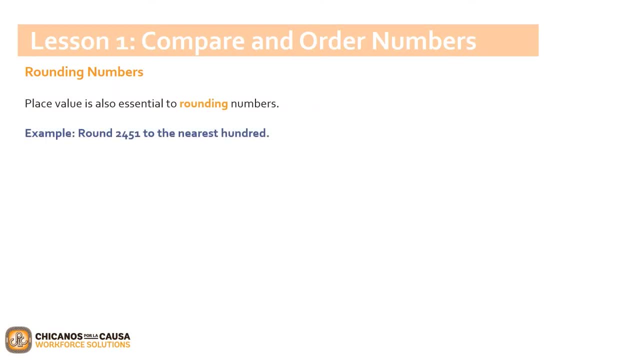 Place value is also essential to rounding numbers. For example, let's round the following number- 2451, to near 100.. First locate the place value that you want to round to. Then look at the place value to the right. 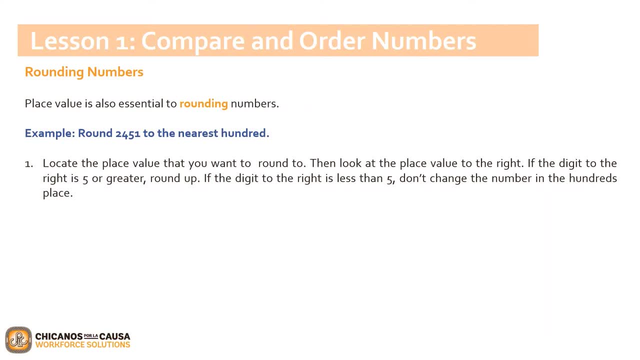 If the digit to the right is 5 or greater, round to the right, greater round up. If the digit to the right is less than five, don't change the number in the hundreds place. So, using our example 2451,, the value to the right of the hundreds place is a. 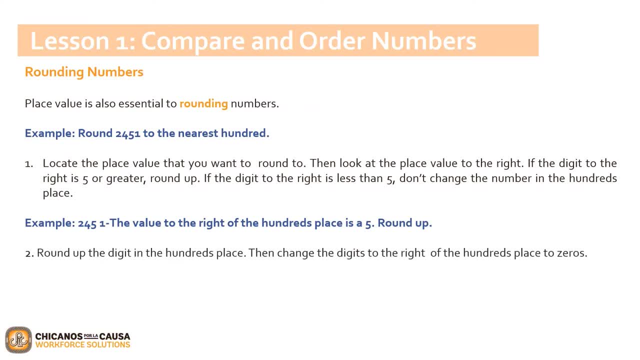 five. Therefore, we would have to round up. Secondly, as I just mentioned, we'd round up the digit in the hundreds place, then change the digits to the right of the hundreds place to zeros. So, using our same example, 2451 would round up to 2,500.. Now that we've gone over compare and 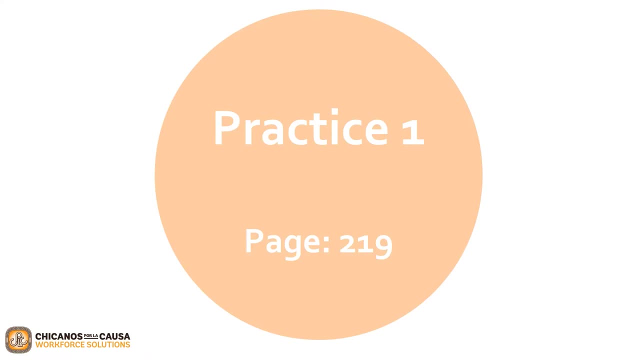 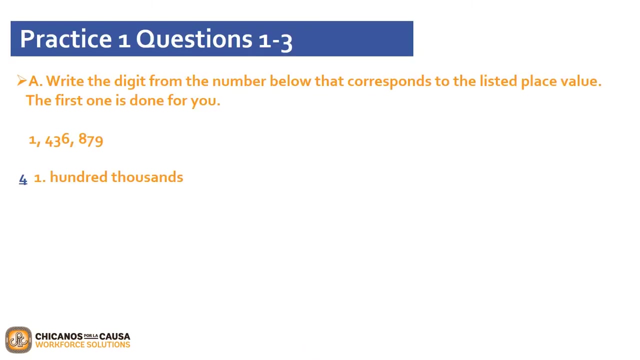 order numbers. let's see our first practice. Practice one found page 219.. For our first practice, we're going to write the digit from the number below that corresponds to the listed place value. The first one is done for you. As you can see, for question one, number four is the corresponding. 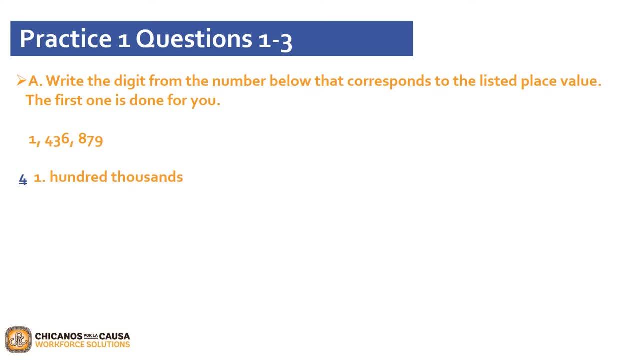 digit to the hundreds thousands place. Question two states hundreds. What digit or number would you write for the hundreds place? The correct digit or number for the hundreds place is eight. Question three: cincoé wheels. What digit or number for the hundreds place? The correct digit or number for the hundreds place is nine. 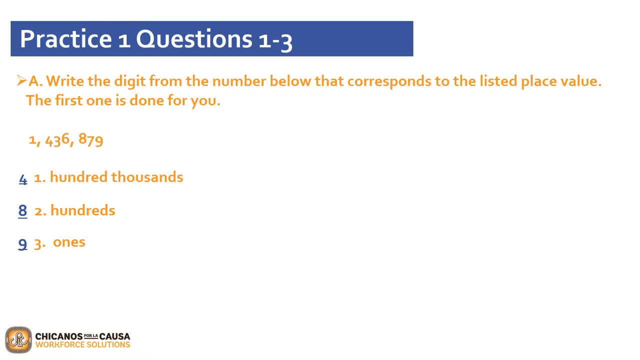 Let me now pause the video and complete questions four through seven. Practice one: find page one: Practice one: find page two: Practice one: find page three: Practice one: find page four: Practice one: find page five: Practice one: find page six: practice 1e, questions 24 to 25.. Click play when you're ready to continue. 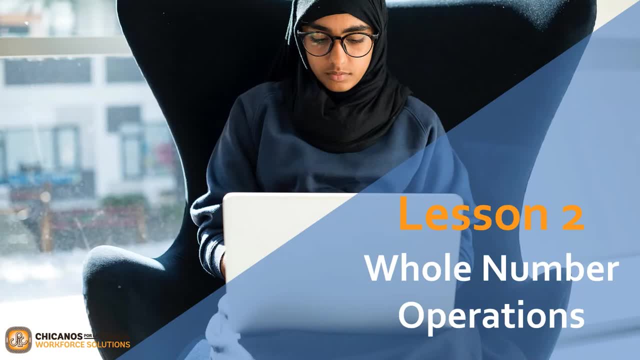 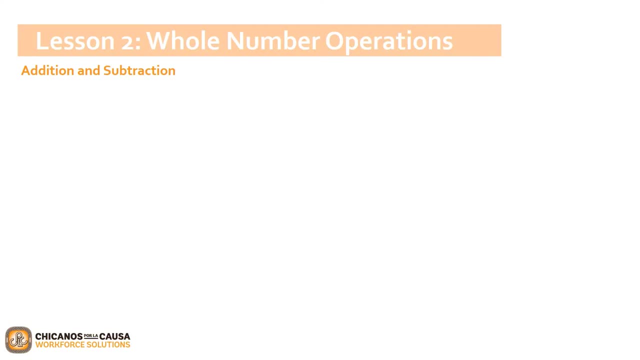 We are now moving on to lesson two: whole number operations. You use addition when you need to combine amounts. The answer in addition problem is called the sum or total. When you are adding, it's helpful to stack the numbers in a column. 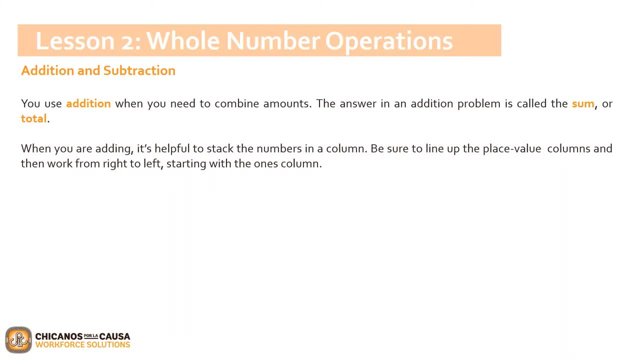 Be sure to line up the place value columns and then work from right to left, starting with the ones column. Sometimes the digits in a place value column add up to 10 or more. When this happens, you can use addition. when you want to combine the numbers, You can also. 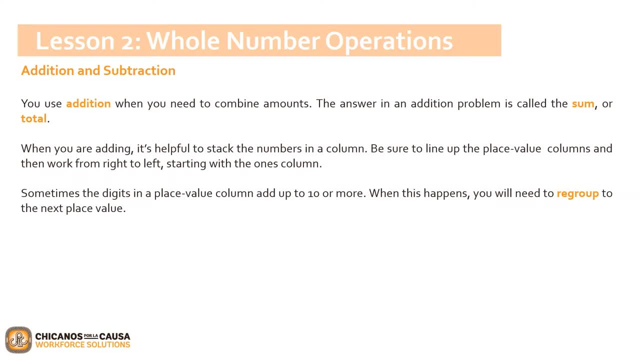 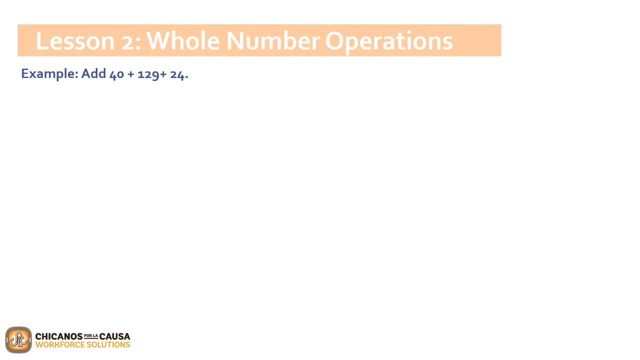 you will need to regroup to the next place value. Let's now take a look at an addition example for Lesson 2.. Our addition example says: add 40 plus 129 plus 24.. First align the numbers you want to add on the ones column. 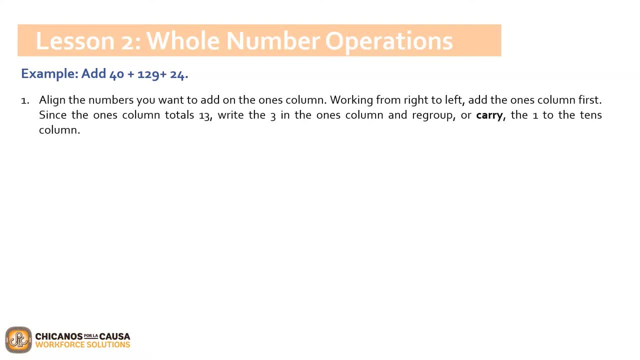 Working from right to left. add the ones column first, Since the ones column total is 13,. write the 3 in the ones column and regroup or carry the 1 to the tens column Second. add the tens column including the regrouped 1.. 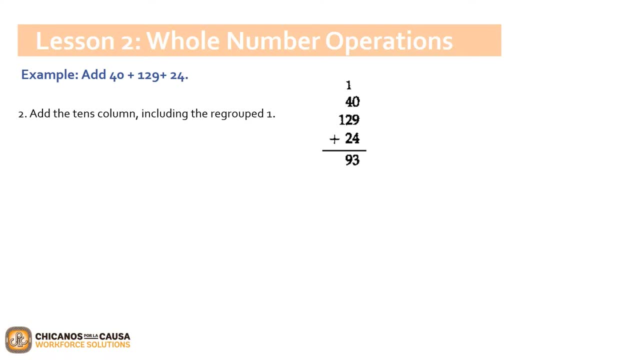 As seen here in our example, we have regrouped or carried the 1 to the tens column and regrouped the 1 to the tens column And now have the number 93.. Third, then add the hundreds column. Since there is only one value, write the 100 in the answer. 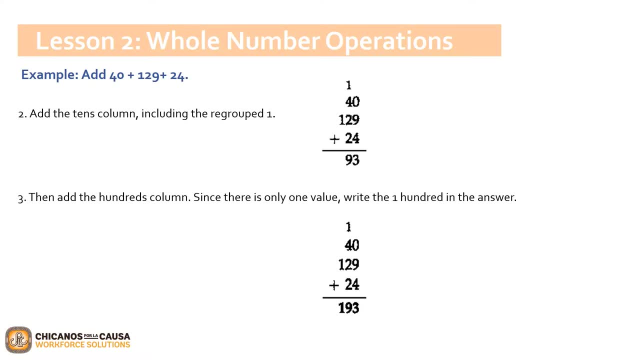 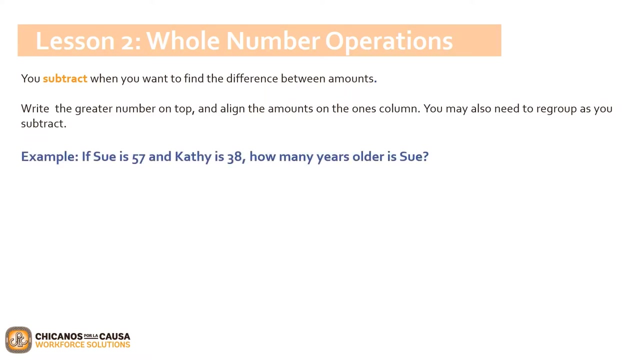 Now our answer is 193.. You subtract when you want to find the difference between amounts, Write the greater number on top and align the amounts on the ones column. You may also need to regroup as you subtract. Our subtraction example says: if Sue is 57 and Kathy is 38, how many years older is Sue? 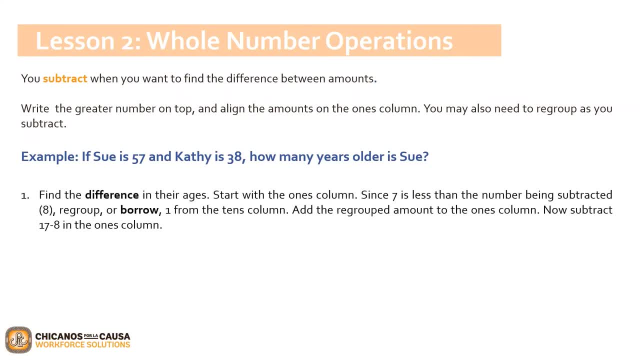 First let's find the difference in their ages. Start with the ones column, Since 7 is less than the number being subtracted 8, regroup or borrow 1 from the tens column. Add the regrouped amount to the ones column. 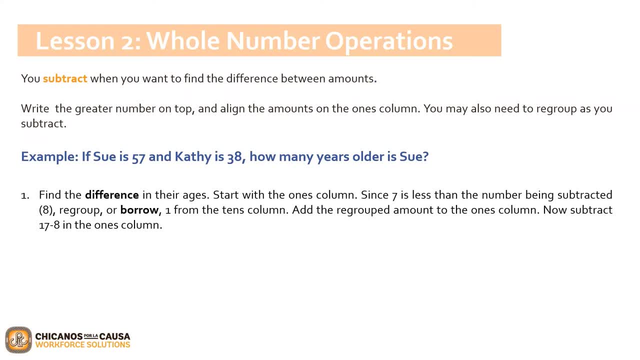 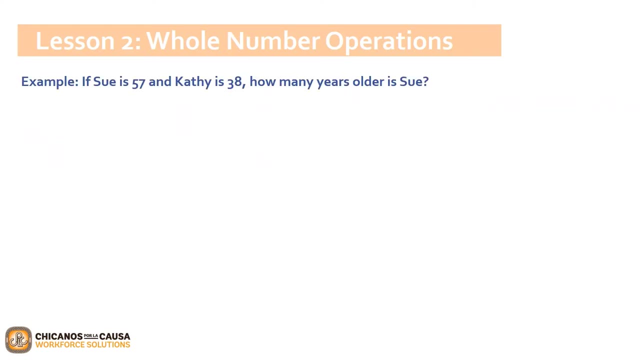 Now subtract 17 minus 8 in the ones column. As you can see, when we subtract 17 minus 8 in the ones column we get 9.. Second, subtract 4 minus 3 and write the result in the tens column of the answer. 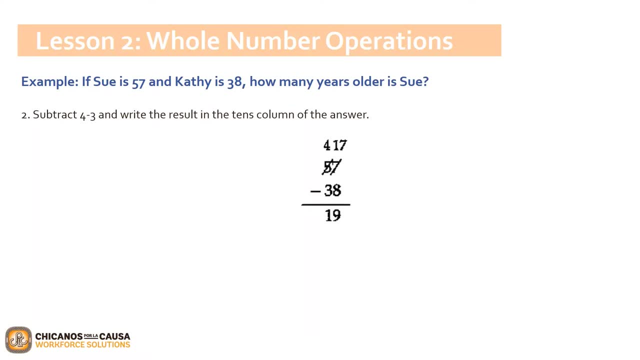 As we can see, if we subtract 4 minus 3 in the tens column, we get 1.. Therefore, our answer for the example is: Sue is 19 years older than Kathy. We can check if our answer is correct by adding 19,. our answer plus 38, Kathy's age, which equals 57, Sue's age. 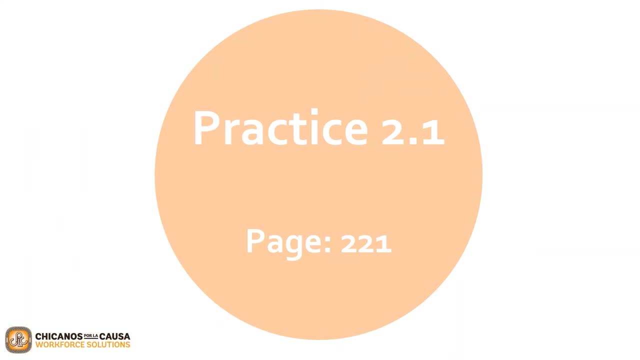 Now that we have finished learning about addition and subtraction, let's go ahead and proceed to practice 2.1, found on page 221.. For the following three questions, we'll be solving either an addition or subtraction problem. Our first question is an addition problem. 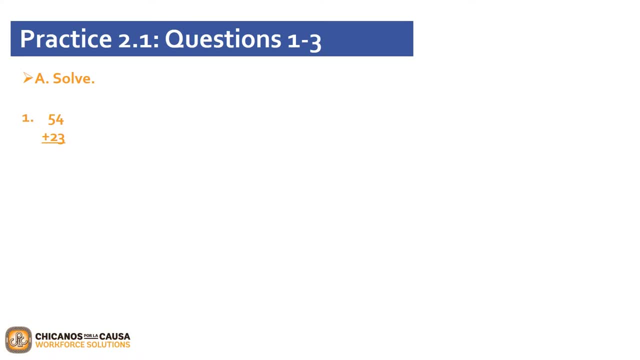 It's asking us to add 54 plus 23.. Based on what we previously learned, how would we solve and answer this question? We would solve this question by adding 4 plus 3 in the ones column and adding 5 plus 2 in the tens column, in which our answer would be 77.. 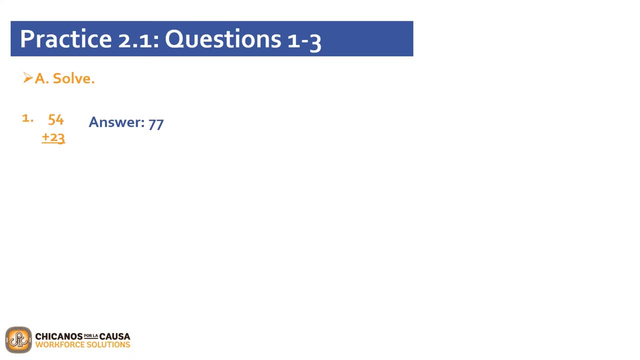 Our second question is another addition problem. It's asking us to add 46 plus 54. How would we solve and answer this question? We would solve this question by adding 6 plus 4 in the ones column and regrouping or carrying the 1 to the tens column. 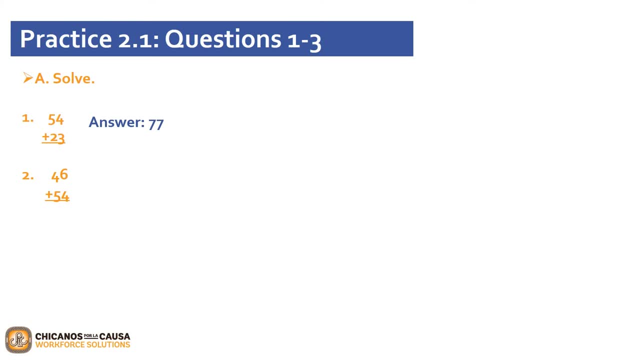 We would then add 1 plus 4 plus 5 in the tens column, Which would give us the answer of 100.. The third question is a subtraction problem. It's asking us to subtract 73 minus 21.. How would we solve and answer this question? 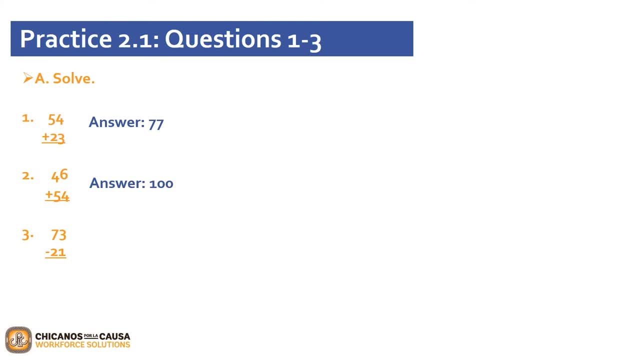 We would solve this question by subtracting 3 minus 1 in the ones column and subtracting 7 minus 2 in the tens column. This would give us the answer of 52.. You may now pause the video and complete questions 4 through 8,, practice 2.1b, questions 9 through 20, and practice 2.1c, questions 21 and 22.. 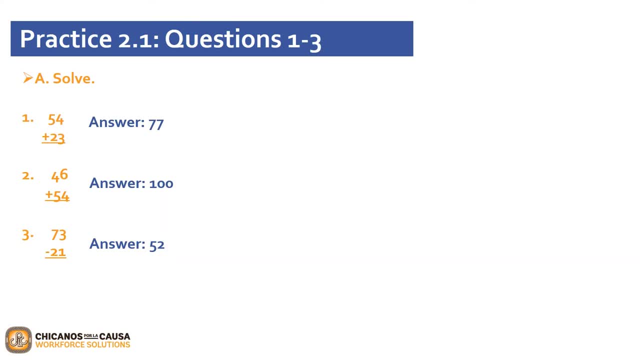 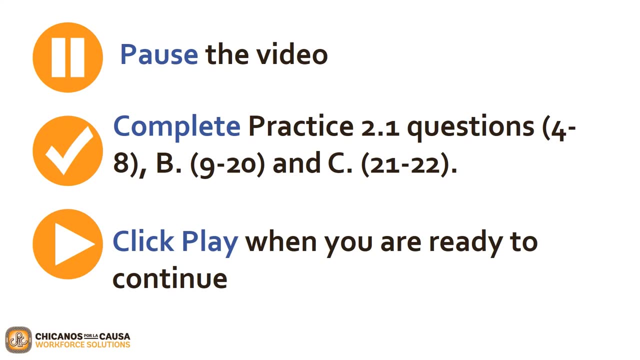 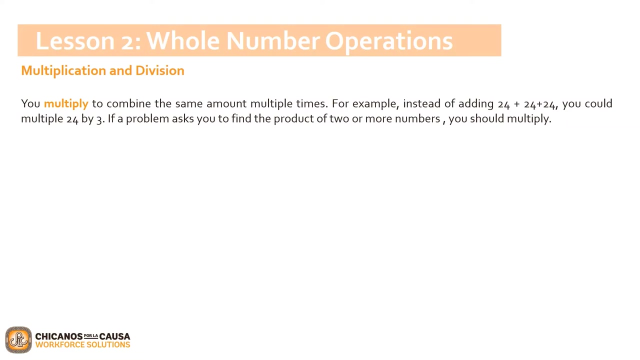 Click play when you're ready to continue. You multiply to combine the same amount multiple times. For example, instead of adding 24 plus 24 plus 24, you could multiply 24 by 3.. If a problem asks you to find the product of two or more numbers, you should multiply. 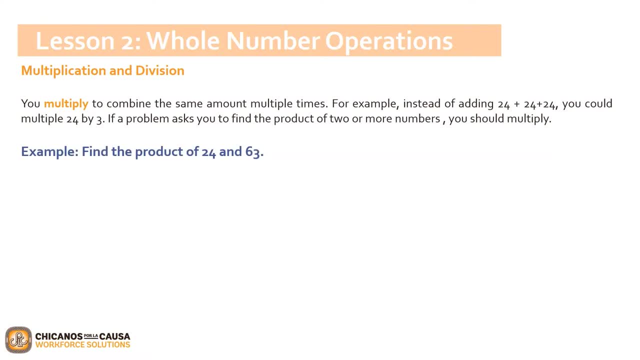 For example, find the product of 24 and 63.. For example, find the product of 24 and 63.. First align place values. as you rewrite the problem in a column, Multiply the ones place of the top number by the ones place of the bottom number. 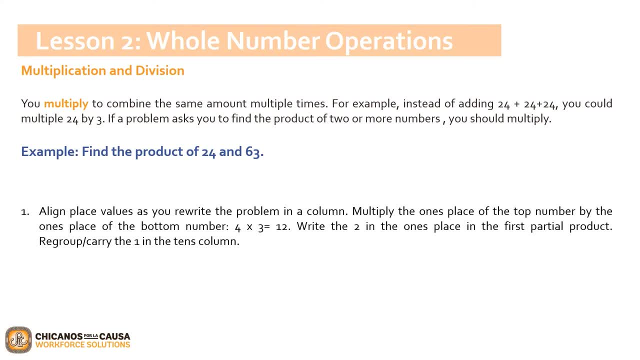 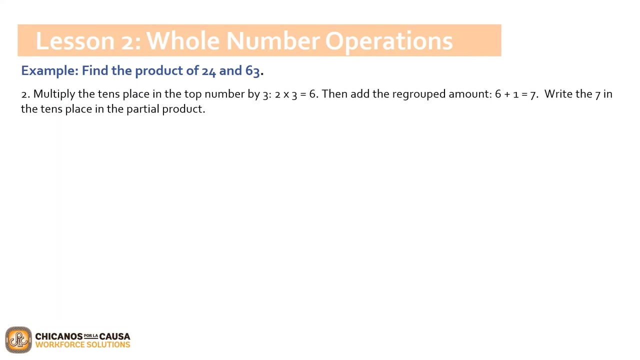 4 times 3 equals 12.. Write the 2 in the ones place in the first partial product. Regroup or carry the 1 in tens column. Multiply the tens place in the top number by 3.. 2 times 3 equals 6.. 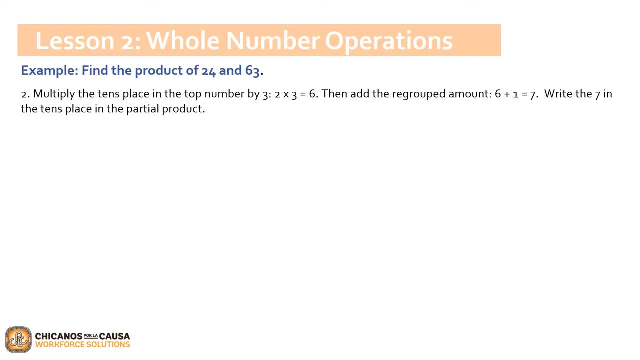 Then add the regrouped amount: 6 plus 1 equals 7.. Write the 7 in the tens place in the partial product. Third, now multiply by the tens place of 63.. Write a placeholder 0 in the ones place in the second partial product. 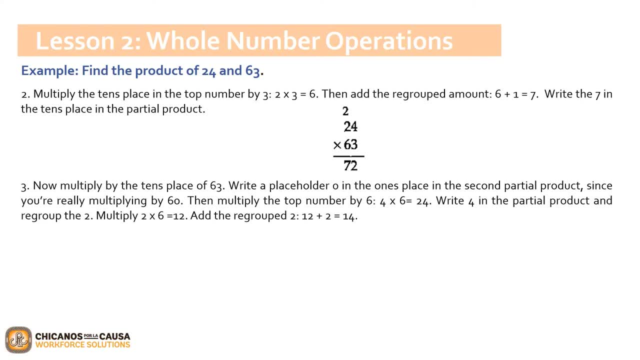 Since you really multiply by 60. Then multiply the top number by 6.. 4 times 6 equals 24.. Write 4 in the partial product and regroup the 2. Multiply 2 times 6, which equals 12.. 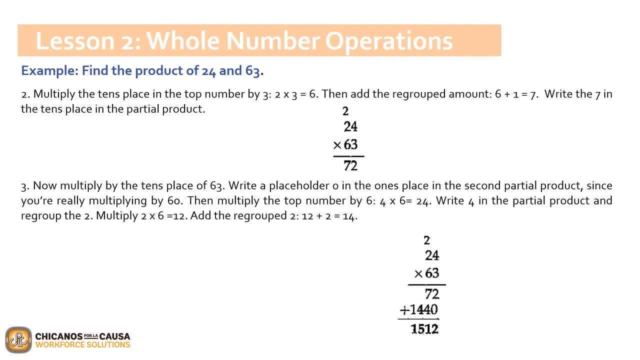 Add the regrouped 2 to 12 plus 2, which equals 14.. Fourth, multiply by the tens place in the tens column. Add the partial products to find the total product. So 72 plus 1,440 equals our answer 1,512. 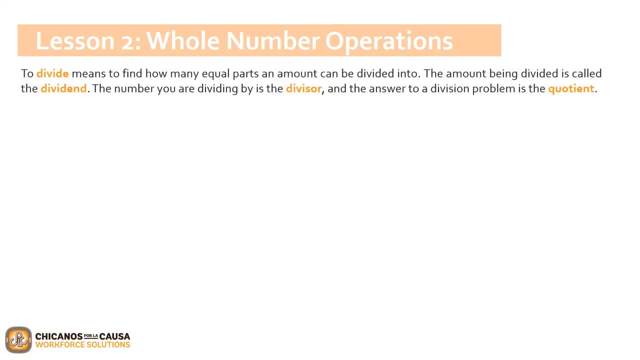 To divide means to find how many equal parts an amount can be divided into. The amount being divided is called the dividend. The number you are dividing by Is the divisor, And the answer to the division problem is the quotient. Here's an example of a division problem. 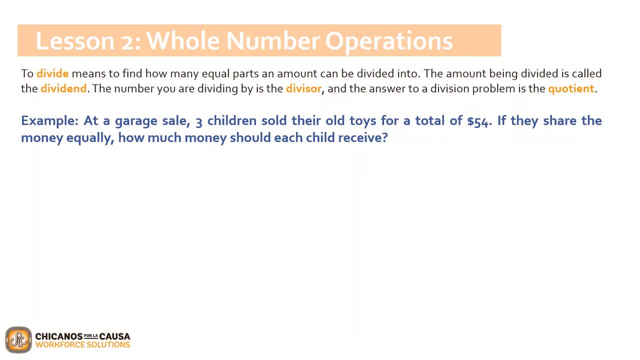 At a garage sale, three children sold their old toys for a total of $54.. If they shared the money equally, how much money should each child receive First? divide the total amount- $54, by the number of ways the money is to be split 3.. 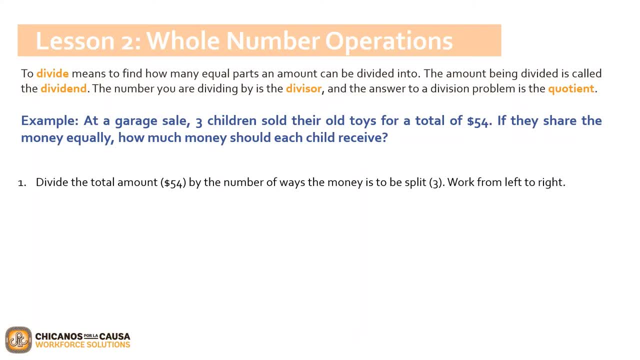 Work from left to right. How many times does 3 go into 5?? Write the answer: 1 directly above the 5 in the dividend, Since 3 times 1 equals 3, subtract 5 minus 3, which equals 2.. 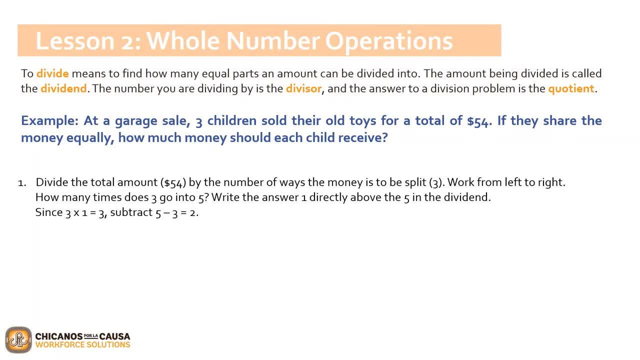 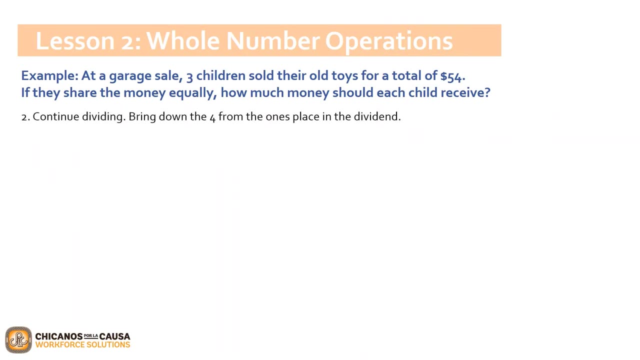 Second, divide the total amount by the number of ways the money is to be divided. The number of ways the money is to be divided is equal to 1.. Write the answer 2 directly above the 4 in the dividend, Since 3 times 1 equals 3, subtract 5 minus 3, which equals 2.. 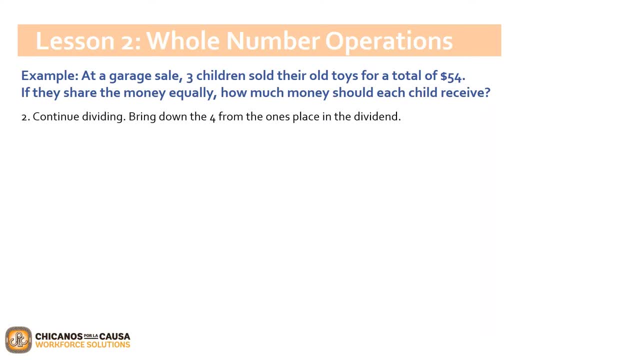 How many times does 3 go into 24?? Write the answer: 2 directly above the 4. in the dividend, Since 3 times 1 equals 3, subtract 5 minus 3,, which equals 2.. in Since 3 times 8 equals 24, subtract 24 minus 24,, which equals 0.. Therefore our answer: 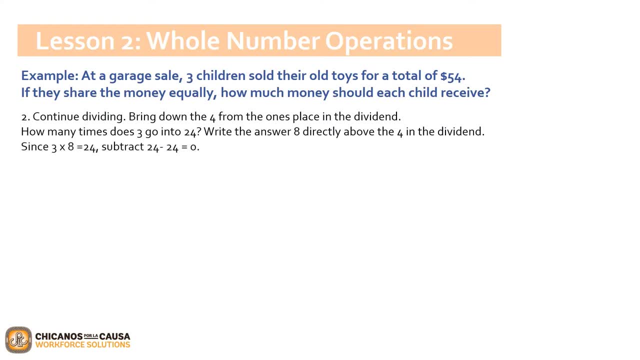 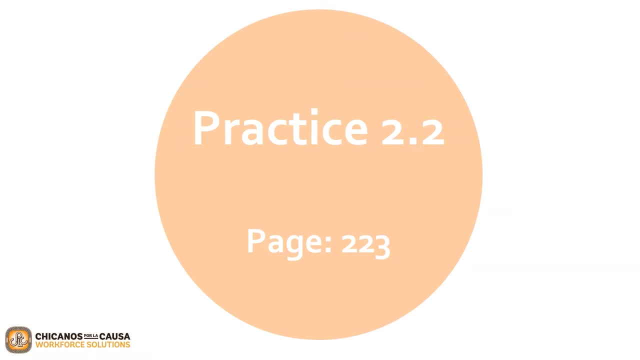 would be, each child should receive 18 dollars. Now that we've covered multiplication and division, let's go ahead and proceed to practice 2.2, found on page 223.. For the following three questions, we will be solving multiplication problems. The first question is asking us to multiply 121. 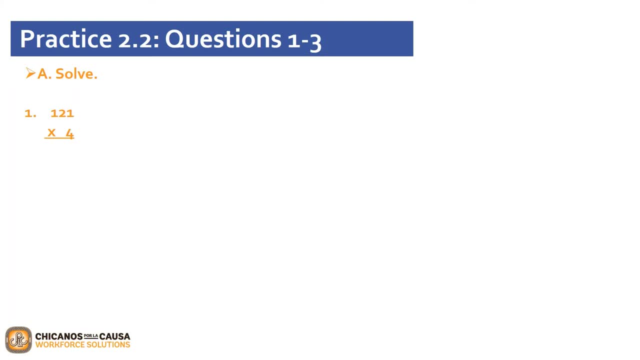 times 4.. Based on what we've previously learned, how could we solve and answer this question? We will solve this question by multiplying 4 times 1 in the ones place, then multiplying 4 times 2 in the tens' place, and then multiplying 4 times 1 in the hundreds' place. This would 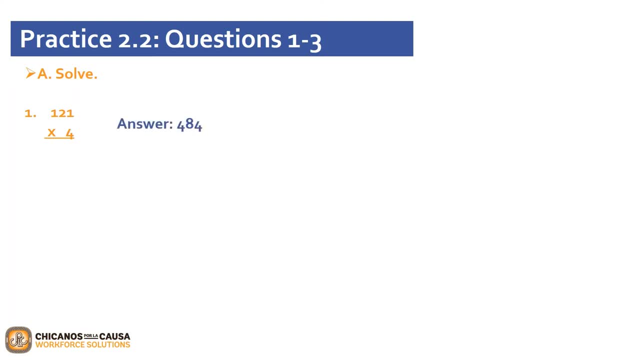 give us our answer of 4.2 times 4.0 times 4.0.. This would give us the answer of 4.0 times 4.0 times. Our second question is asking us to multiply 250 times 4.. 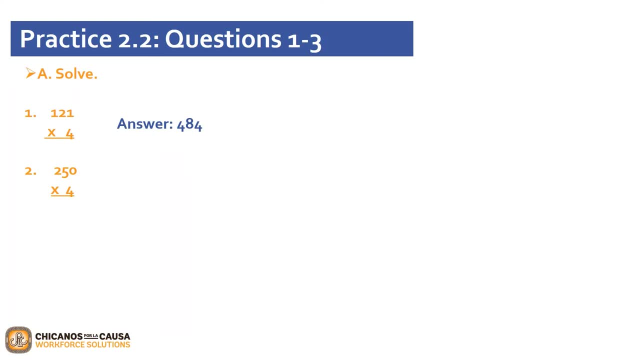 How would we solve and answer this question? We would solve this question by multiplying 4 times 0 in the ones place, then multiplying 4 times 5 in the tens place and then multiplying 4 times 2 in the hundreds place. 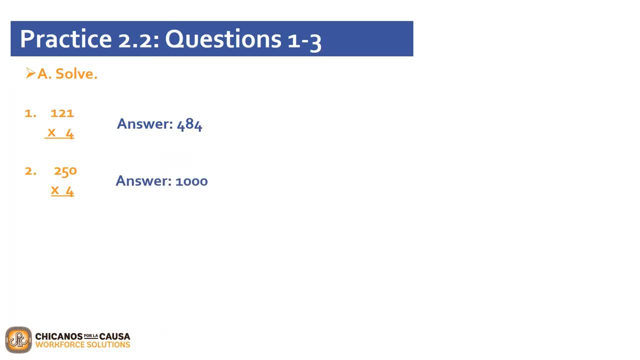 This would give us our answer of 1000.. The third question is asking us to multiply 342 times 8.. How would we solve and answer this question? We would solve this question by first multiplying 8 times 2, which equals 16.. 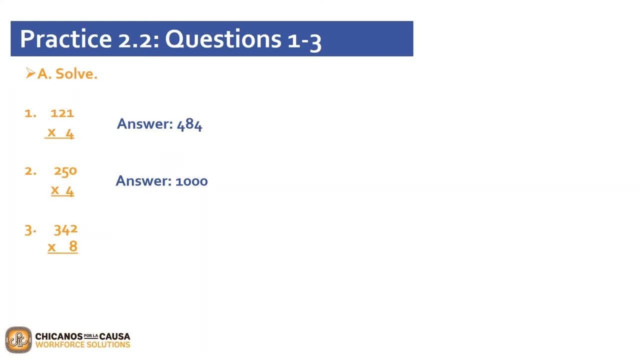 We would regroup or carry the 1 from 16 in tens place. Then we would multiply 4 times 8 plus 1 in the tens place, tens place, which equals to 33.. We would regroup or carry the 3 from 33 in the hundreds place. 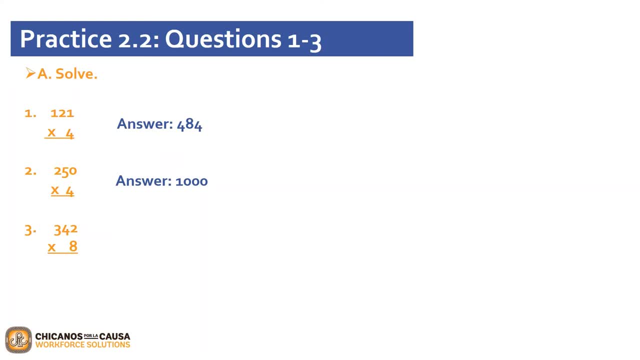 Afterwards, we would multiply 8 times 3 plus 1 in the hundreds place, in which our answer would be 2736.. You may now pause the video and complete questions 4 through 12, practice 2.2b, questions 13 through 21,. practice 2.2c, questions 22 to 23, and practice 2.2d, question 24.. 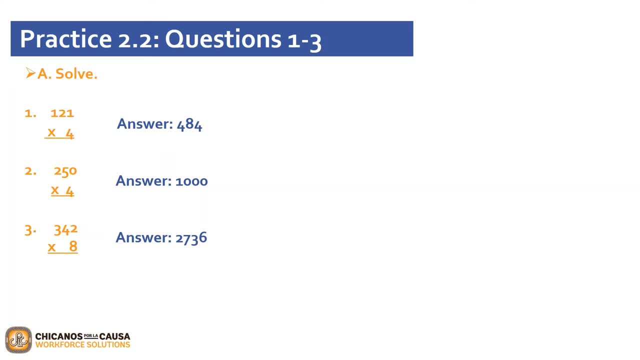 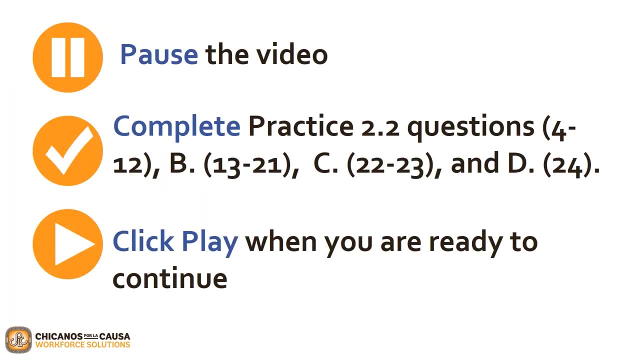 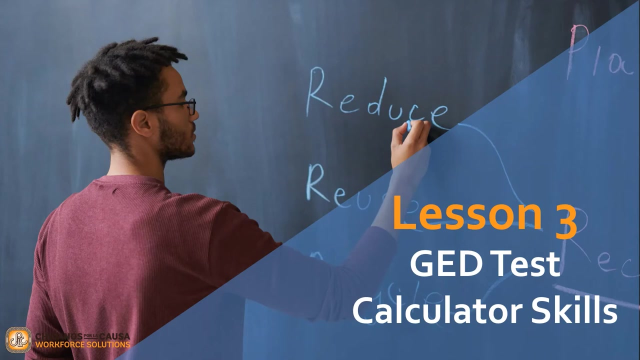 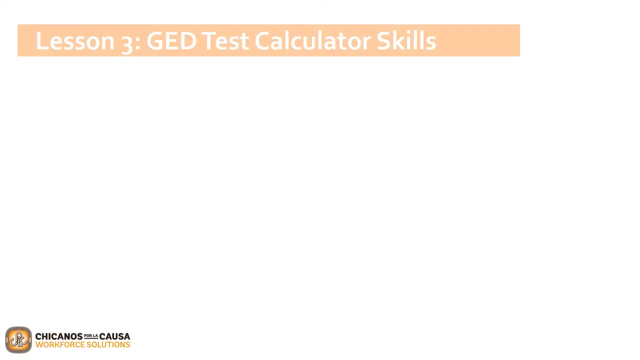 Click play when you're ready to continue Phew. Lesson 2 was a long one. Now let's move ahead to Lesson 3, GED Test Calculator Skills. You will have access to an online or handheld calculator for many questions on the Mathematical. 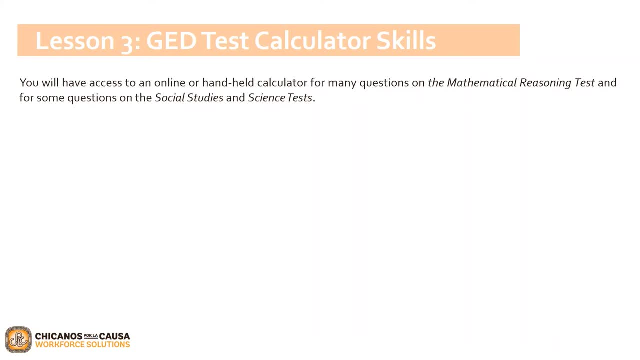 Reasoning Test and for some questions on the Social Studies Test. If you wish to use a handheld calculator, you will likely need to bring your own. The calculator must be the Texas Instruments TI-30XS MultiView. The online version will be available when the calculator icon appears at the top of the computer screen. 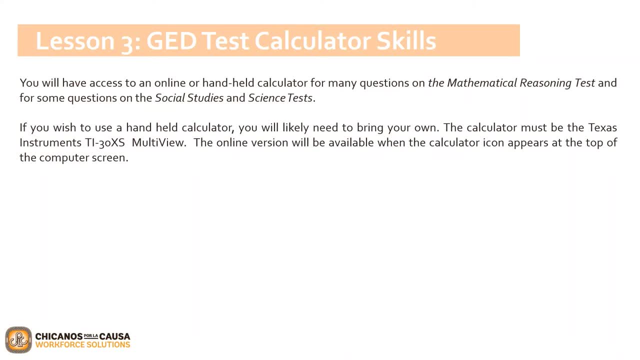 You will click on the icon to open the calculator and use the mouse to move it so that it does not cover the problem. Please use the calculator when you think it will score a point. The calculator will save you time or improve your accuracy when taking the test. 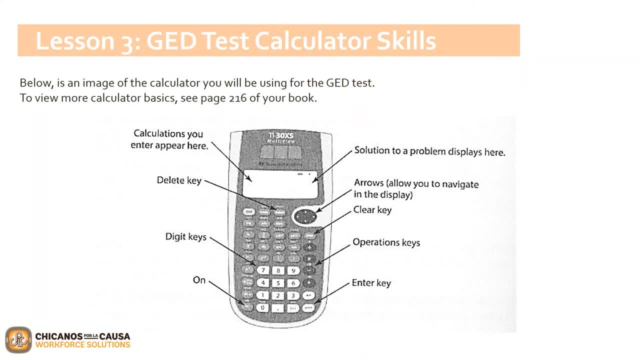 Below is an image of the calculator you will be using for the GED test. To view more calculator basics, please click the link in the description: See page 216 of your book. Now let's view an example that demonstrates how to use the calculator's operation keys. 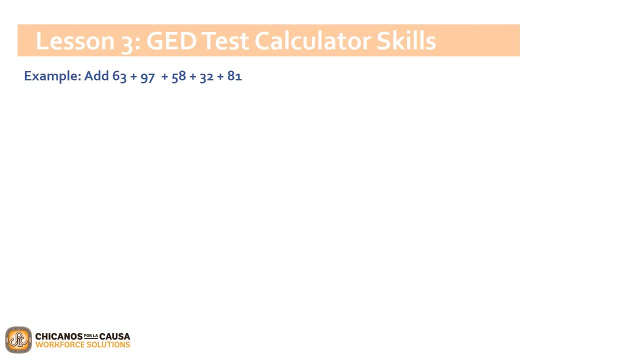 Our example to practice our calculator skills says: Add 63 plus 97 plus 58 plus 32 plus 81.. First always clear your calculator before starting a new computation. On the TI-30XS MultiView, use the clear key. 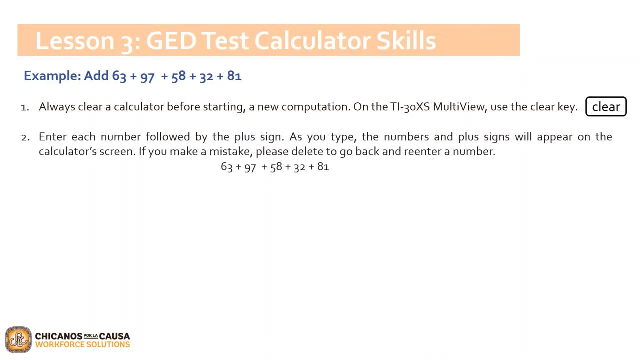 Second, enter each number followed by the plus sign. As you type, the numbers and plus signs will appear on the calculator screen. If you make a mistake, please delete to go back and re-enter a number. Third, press enter to find the total. 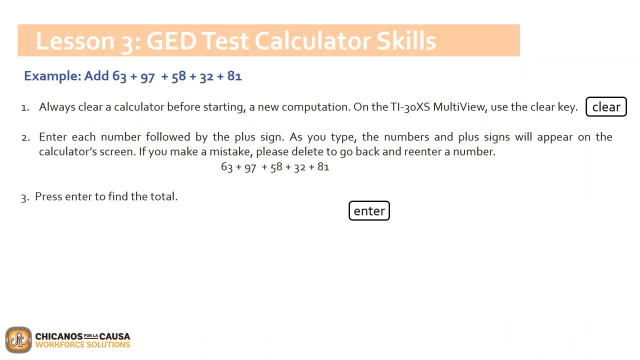 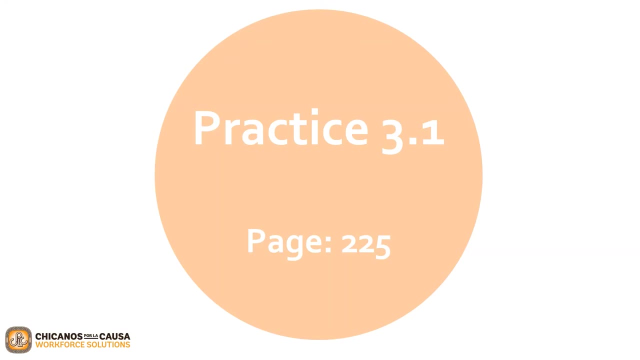 The total 331, will appear on the right-hand side of the display. The total 331, will appear on the right-hand side of the display. Now that we gained new calculator skills, let's move forward to practice 3.1, found on page 225. 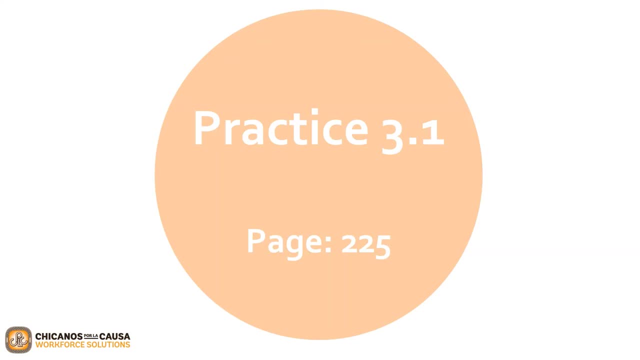 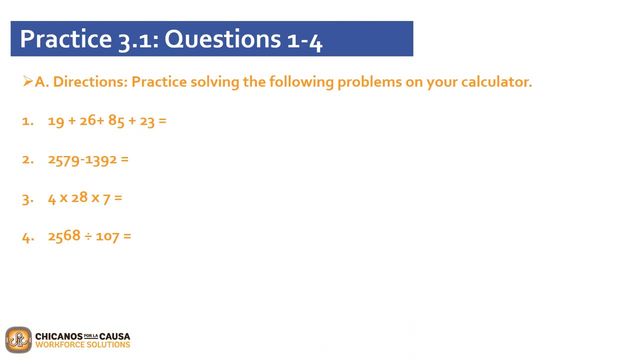 Now that we gained new calculator skills, let's move forward to practice 3.1, found on page 225.. For the following four questions, we'll practice solving math problems using the TI-30XS Multiview Calculator. Question 1 asks us to solve the following addition problem: 19 plus 26 plus 85 plus. 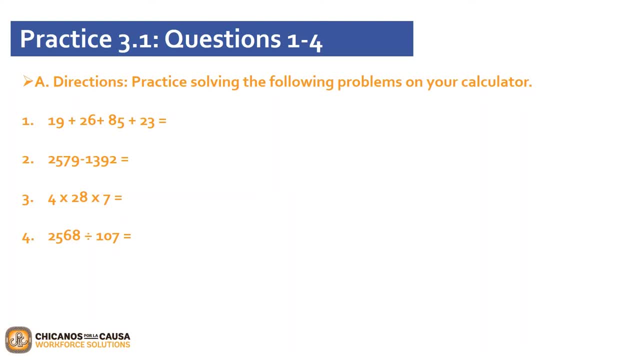 23.. The answer for this question is 153.. Question 2 asks us to solve the following subtraction problem: 2,579 minus 1,392.. The answer for this question is 1,187.. Question 3 asks us to solve the following multiplication problem: 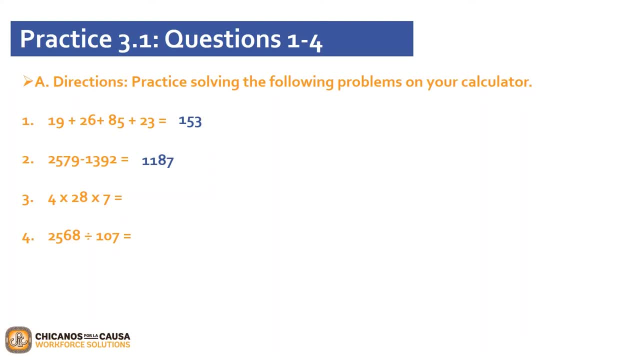 4 times 28 times 7.. The answer for this question is 784.. Question 4 asks us to solve the following division problem: 2,568 divided by 107.. The answer for this question is 24.. You may now pause the video and complete the question. 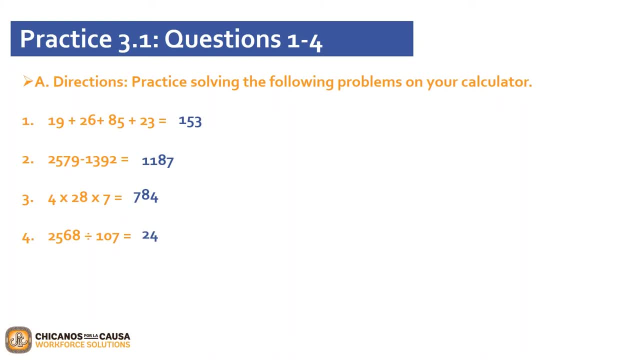 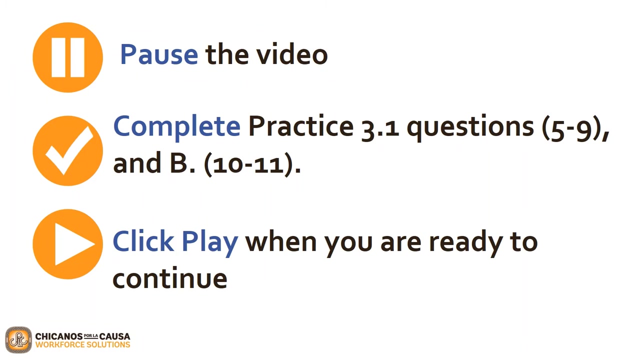 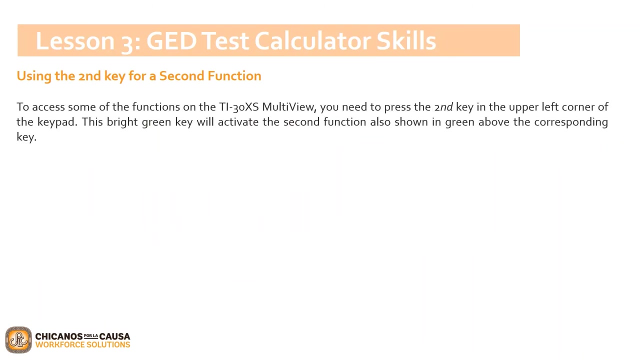 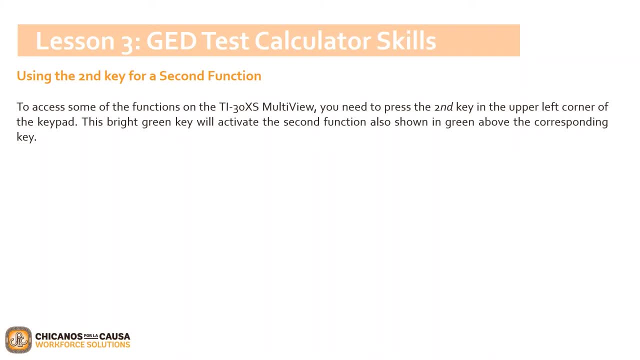 in the upper left corner of the keypad. Yes will activate the second function, also shown in the green above the corresponding key. To access the second function of a key, press the second key first. Do not press it at the same time as the function key. 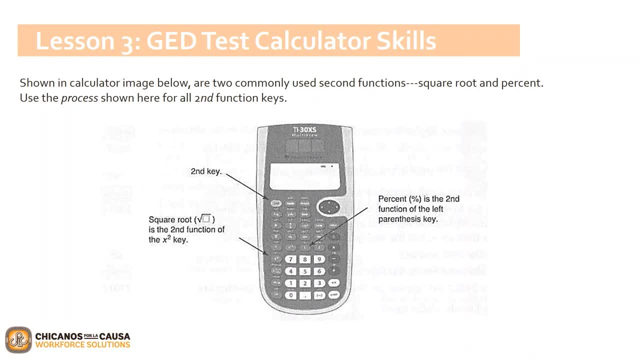 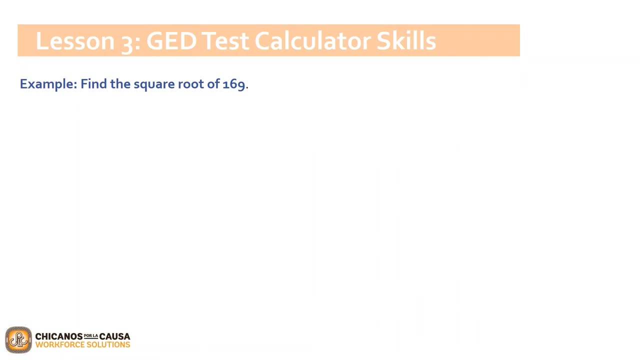 Shown in the calculator image below are two commonly used second functions: square root and percent. Use the process shown here for all second function keys. Now let's view an example that demonstrates how to use the calculator's second function keys. Using our calculator, let's find the square root of 169.. 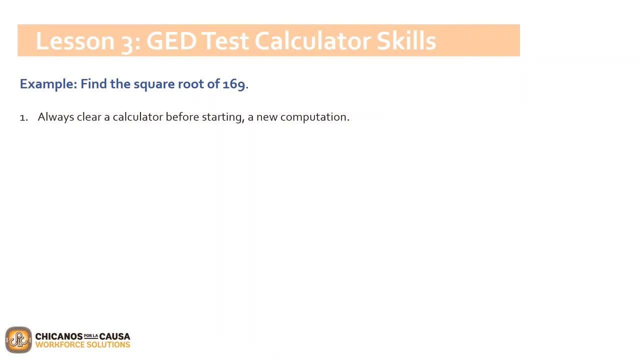 First, always clear a calculator before starting a new computation. Second, recognize that square root is a second function over the x squared key. Press the second key. Note that the term second now appears in the upper left corner of the display. Third: next, press the x squared key to activate the square root function in green over the 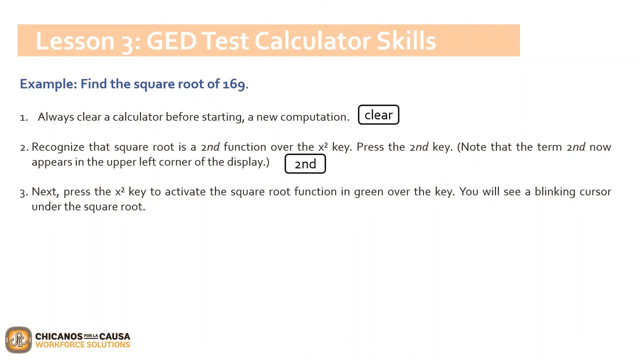 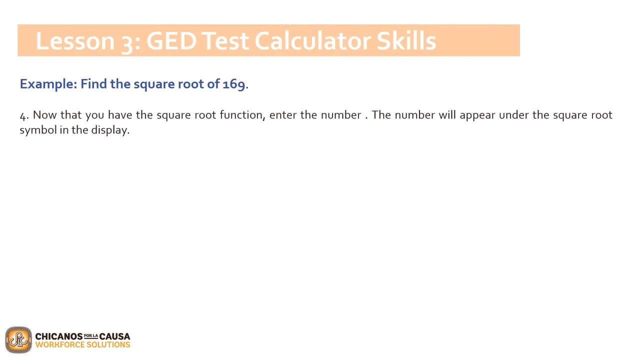 key, You will see a blinking cursor under the square root. Fourth, now that you have the square root function, answer the number. The number will appear under the square root symbol on the display. Fifth, press the answer key to find the square root. The answer 13 will appear on the right-hand side of the display. 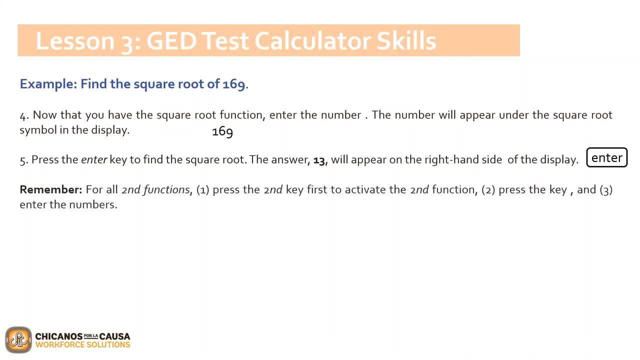 Remember, a square root is a second function over the square root. What do you mean For all second functions? press the 2nd key first to activate the second function. 2nd, press the key and 3rd, enter the numbers. 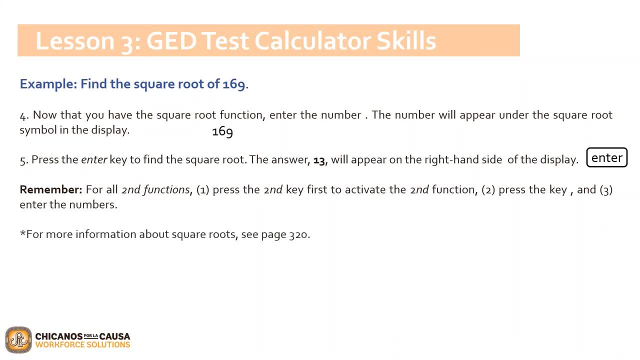 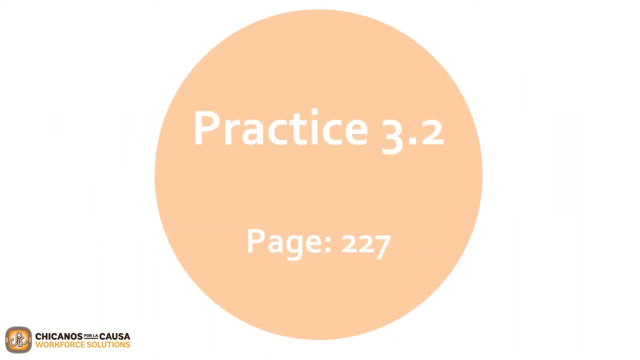 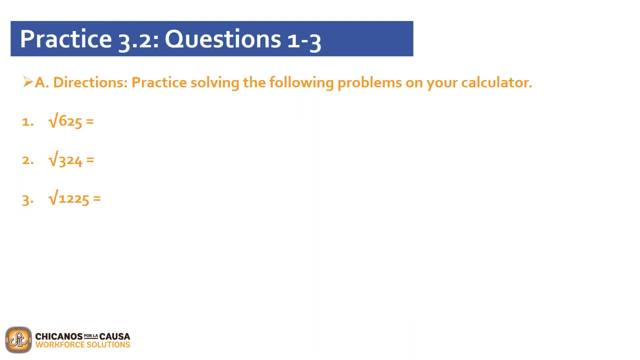 For more information about square roots, see page 320.. Now that we learned more about how to use the second function keys, let's do practice 3.2, found on page 227.. As we previously did for practice 3.1,. 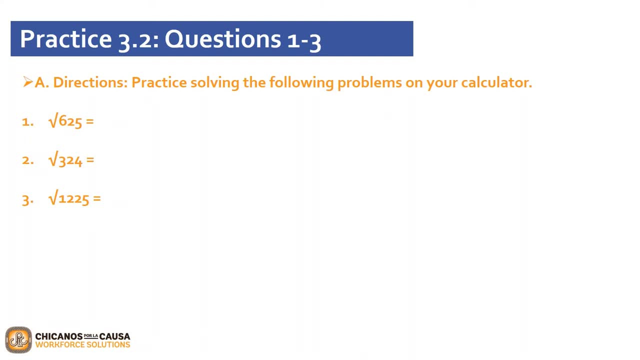 we will practice solving math problems using the TI-30XS multi-view calculator. Question 1 asks us to solve the following square root problem: What is the square root of 625?? The answer for this question is 25.. Question 2 asks us to solve the following problem: 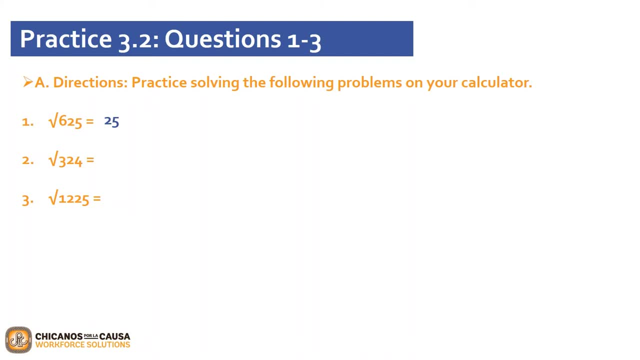 What is the square root of 324?? The answer for this question is 18.. Question 3 asks us to solve the following square root problem: What is the square root of 1225?? The answer for this question is 35.. You may now pause the video and complete questions 4 through 9,. 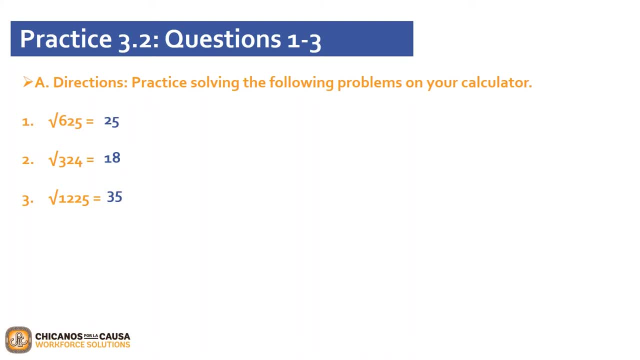 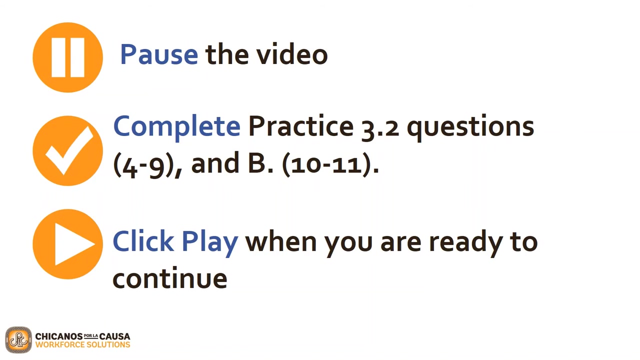 and practice 3.2b questions 10 and 11.. Click play when you're ready to continue. Let's now jump into practice. 3.2b questions 10 and 11.. Let's now jump into practice. 3.2b questions 10 and 11.. 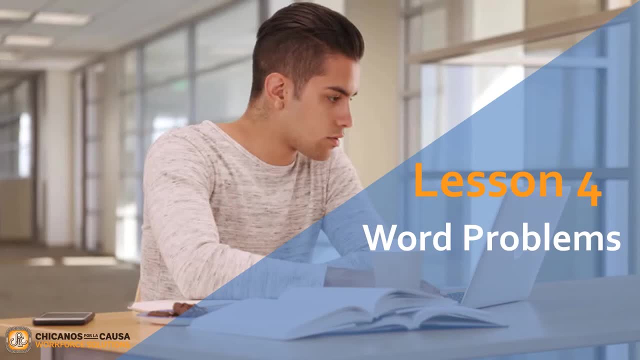 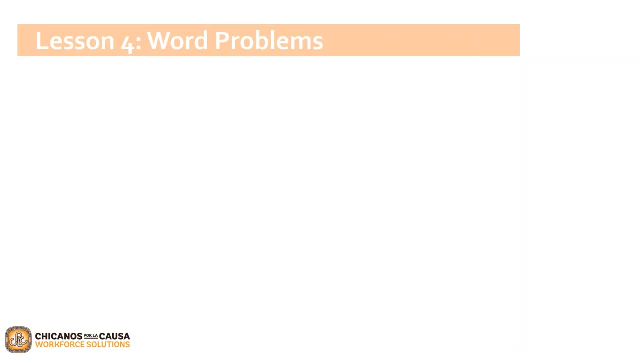 Let's now jump into practice 3.2b, questions 10 and 11.. Let's now jump into lesson 4, word problems. To pass the mathematical reasoning test, you will need to solve word problems. These questions are easier to manage if you use a 5-step problem-solving process. 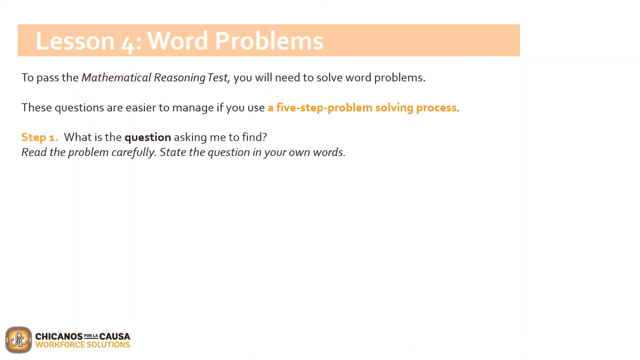 Step 1.. What is the question asking me to find? Read the problem carefully. State the question in your own words: Step 2. What information from the problem do I need? Select only the information you need to answer the question. Step 3. Which operation do I need to perform? Addition, subtraction, multiplication or division? 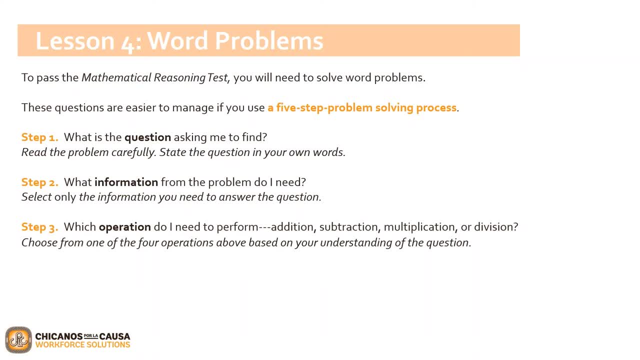 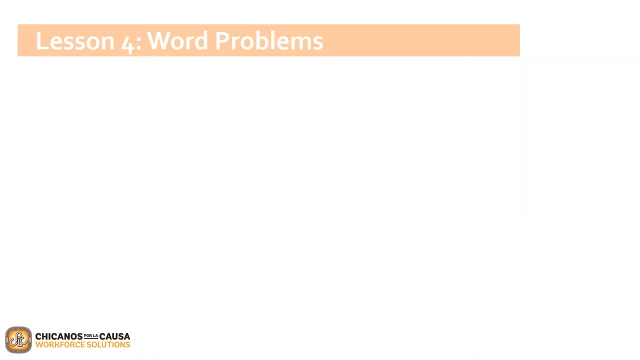 Choose from one of the four operations above based on your understanding of the question. Step 4. What is my solution? Carry out the operation with the numbers you chose in step 2.. Step 5. Does my answer make sense? Look back to make sure that you answered the question. 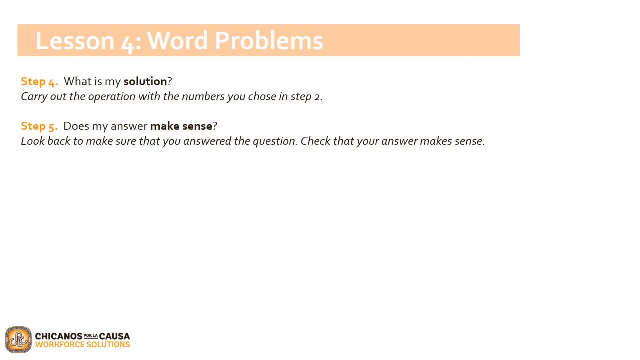 Check that your answer makes sense. To help you decide which operation to use, keep the following ideas in mind: You add in order to combine amounts of different sizes. You subtract in order to find the difference between amounts. You multiply in order to combine the same amount multiple times. 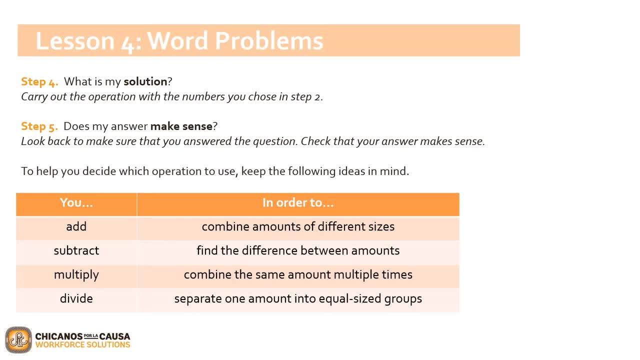 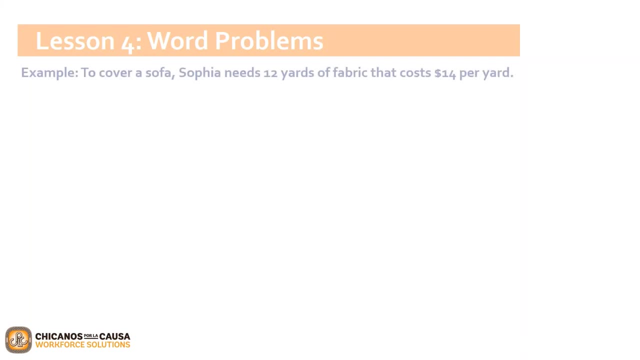 You divide in order to separate one amount into equal-sized groups. Now let's view an example of a word problem. The following word problem says: To cover a sofa, Sophia needs 12 yards of fabric that costs $14 per yard. How many yards does Sophia need for three sofas? 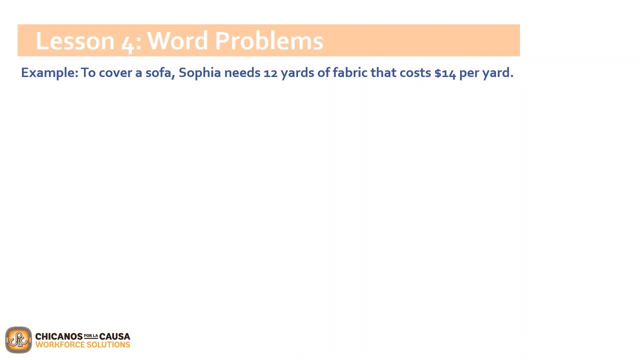 Would it be A 4,, B 36,, C 42, or D 168?? Please feel free to pause the video and take a couple of minutes to solve this problem. Once you're ready to begin again, please click play. 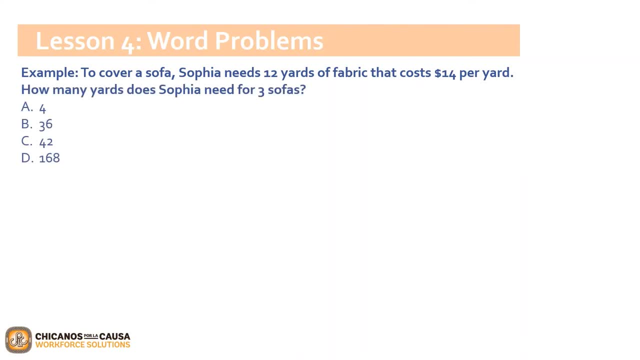 The correct answer for this question is B 36 yards of fabric. The question asks you to find the total number of yards of fabric Sophia needs for three sofas. Note that the cost of a yard of fabric is not needed to answer the question. 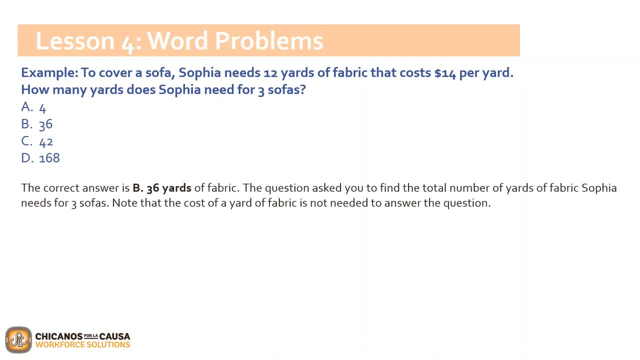 Since you were asked to find the amount of fabric for three sofas, you should have multiplied 12 yards times three sofas, which equals 36 yards. Here are two common errors to avoid. If you had mistakenly divided, you would have gotten the incorrect answer of 4 yards of fabric for three sofas. 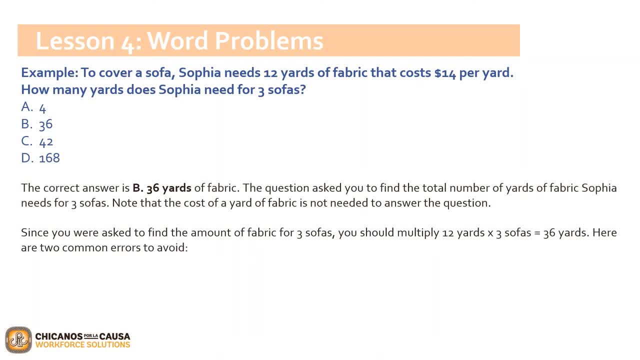 If you had used the $14 price per yard and multiplied by either 3 sofas or 12 yards, you would have been tempted by wrong answers: 42 or 168.. However, the cost per yard is not needed Now that we have reviewed the five-step problem-solving process. 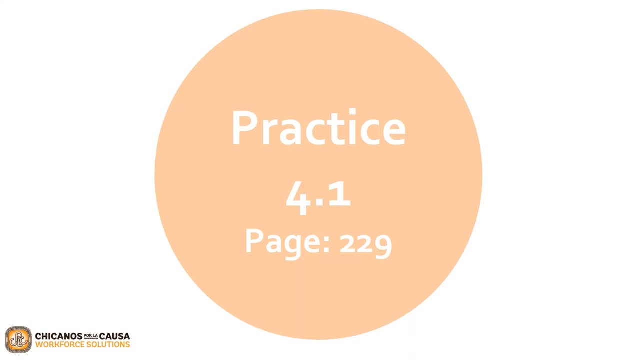 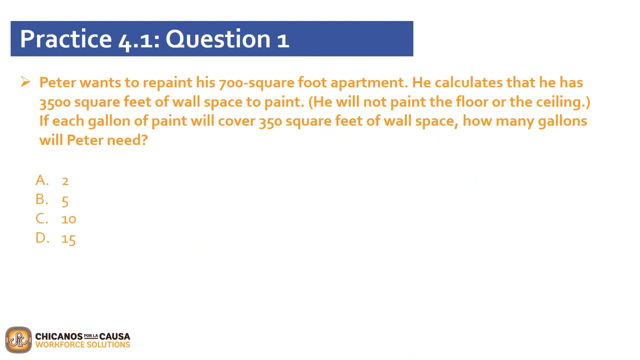 let's move on to practice 4.1, found on page 229.. For practice 4.1, question 1,, we have the following word problem. It reads: as Peter wants to repaint his 700-square-foot apartment, He calculates that he has 3,500 square feet of wall space to paint. 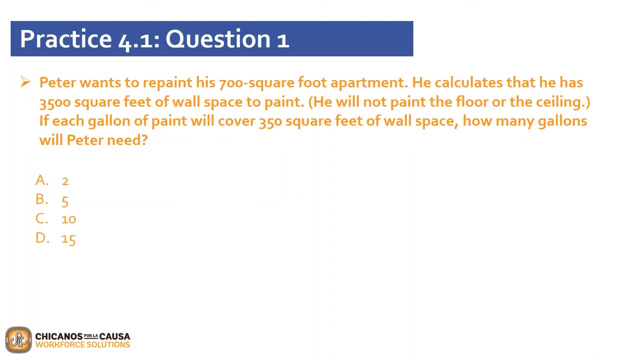 He will not paint the floor or the ceiling. If each gallon of paint will cover 350 square feet of wall space, how many gallons will Peter need? Would it be A, 2,, B 5,, C 10, or D 15?? 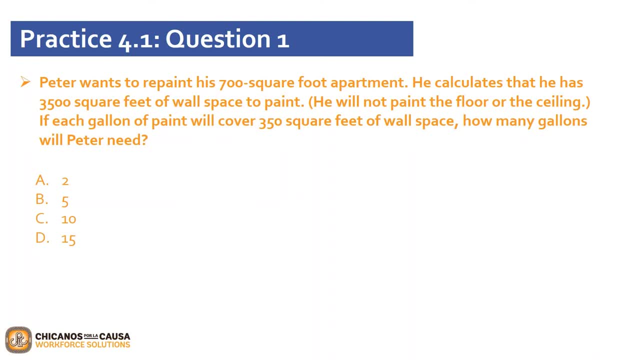 Please feel free to pause the video and take a couple minutes to solve and answer this question. Once you're ready to begin again, please click play. The answer for this question would be C 10.. No paint is needed for the floor, so ignore the 700 square feet. 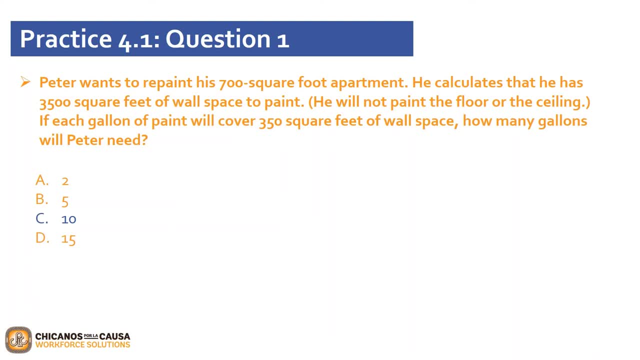 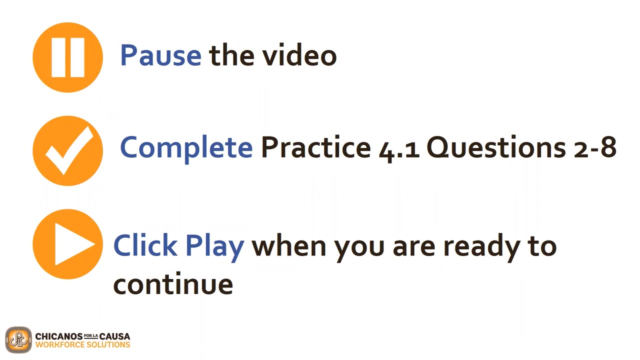 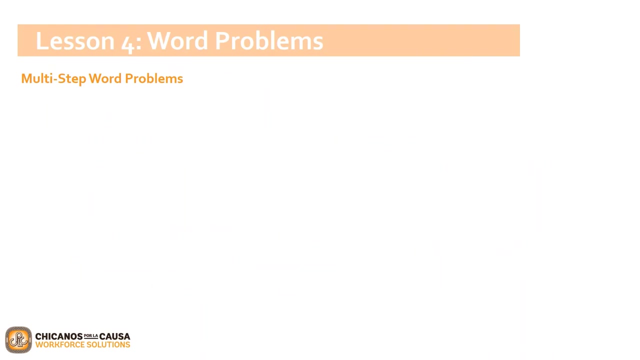 3,500 square feet of wall space divided by 350 square feet per gallon equals our answer of 10 gallons. You may now pause the video and complete questions 2 through 8.. Click play when you're ready to continue. We have previously done word problems that are only one operation to solve. 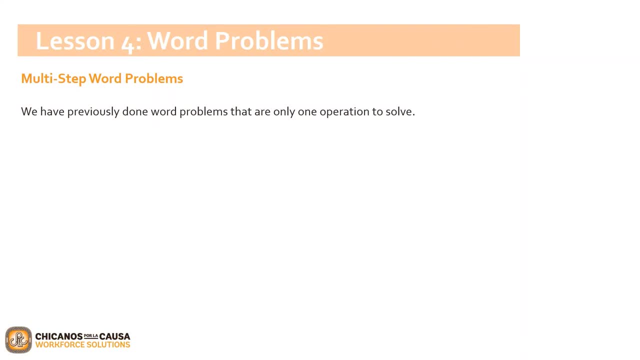 However, on the GED mathematical reasoning test and other tests, you may need to do several math processes to solve a problem. These are called multi-step problems. When you are working on multi-step problems, there are two important ideas to keep in mind. 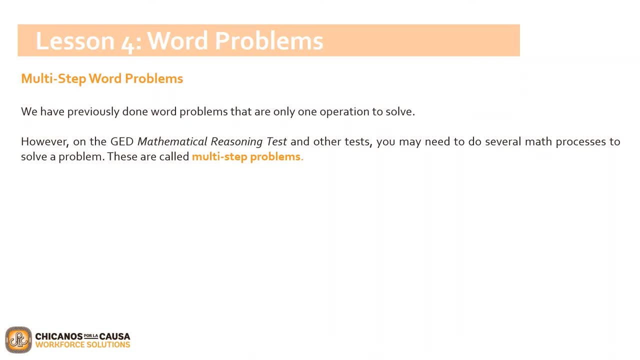 First is what is the question asking me to find? And secondly, did I answer the question? Now let's give an example of a multi-step word problem. Let's call up a teacher Instead of making Richard measure the distance between the people. 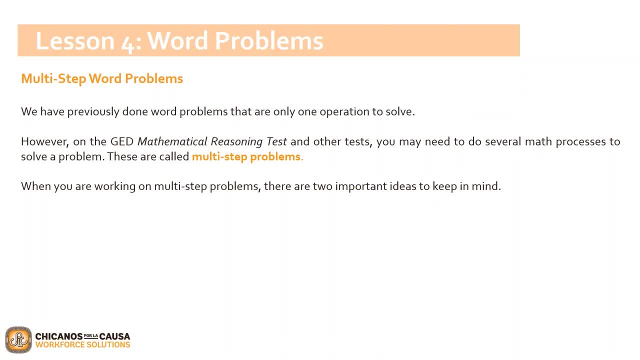 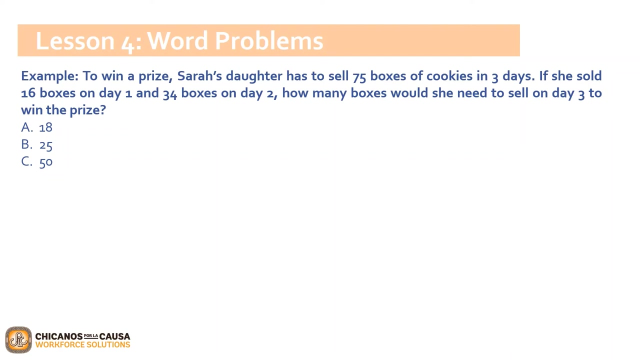 and the teacher and tablet. let's say cool. The following multi-step word problem says: To win a prize, Sarah's daughter has to sell 75 boxes of cookies in 3 days. If she sold 16 boxes on day 1 and 34 boxes on day 2, how many boxes would she need to? 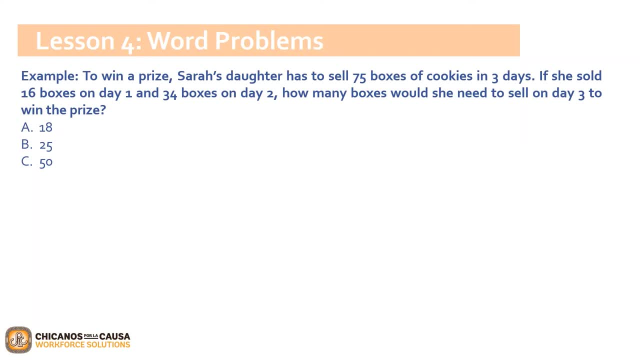 sell on day 3 to win the prize. Would it be 1,, 18,, 2,, 25, or 3, 50?? To solve this problem, step 1 would be: What is the question asking me to find? 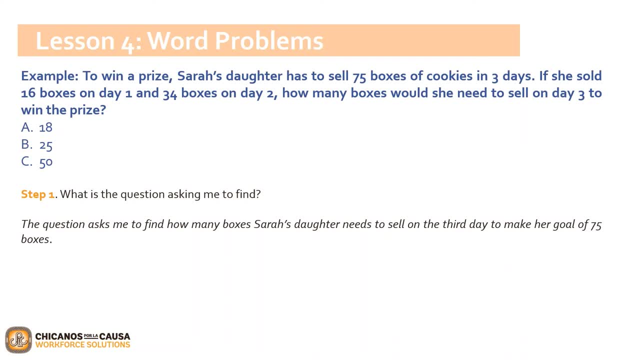 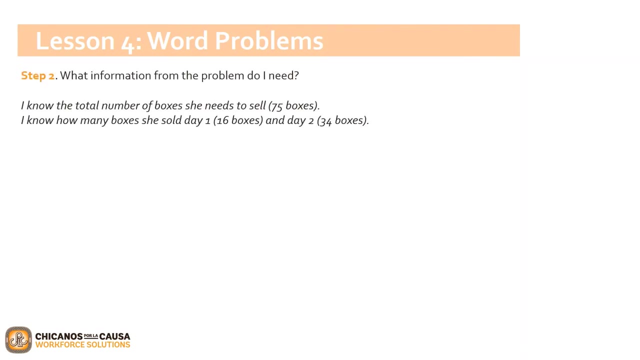 The question asks me to find how many boxes Sarah's daughter needs to sell on the third day to make her goal of 75 boxes, Step 2.. What information from the problem do I need? I know the total number of boxes she needs to sell: 75 boxes. 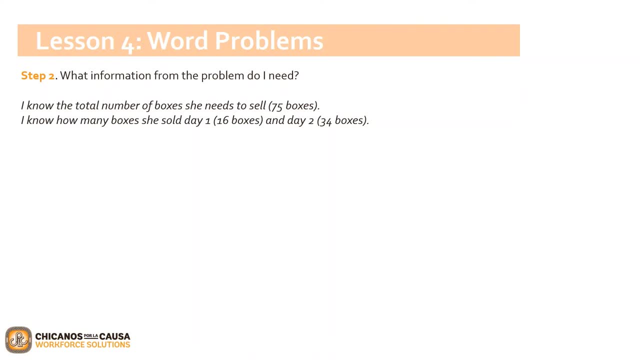 I know how many boxes she sold: day 1, 16 boxes and day 2, 34 boxes. Step 3. Do I need to do only one operation or do I need to do more than one? I can add to find how many boxes Sarah's daughter has sold so far. 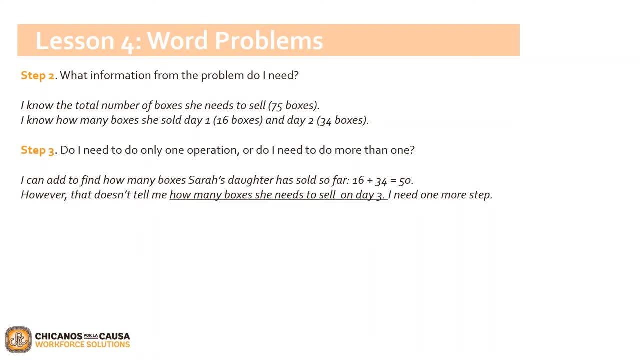 16 plus 34 equals 50. However, that doesn't tell me how many boxes she needs to sell on day 3.. I need one more step, Step 4.. What is my solution? 75 boxes total minus 50 boxes sold equals 25 boxes for day 3.. 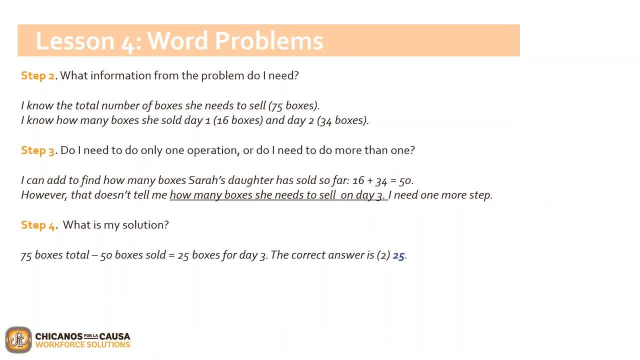 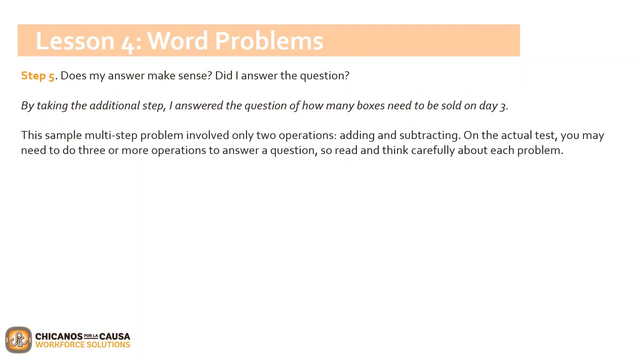 The correct answer is 2, 25.. Step 5.. Does my answer make sense? Did I answer the question By taking the additional step? I answered the question of how many boxes need to be sold on day 3.. This sample multi-step problem involved only two operations: adding and subtracting. 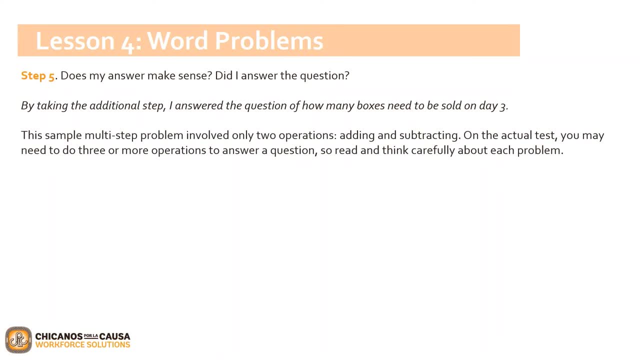 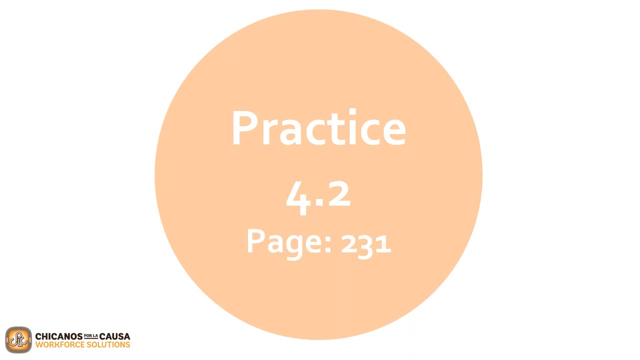 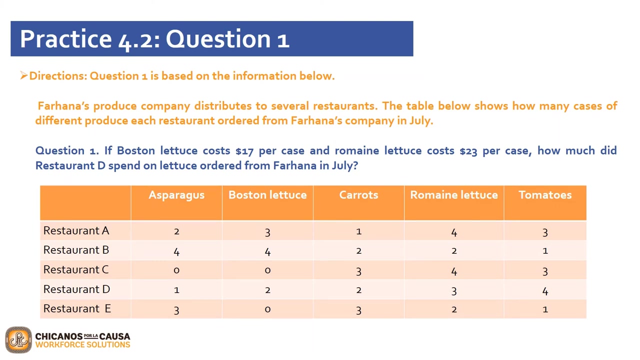 On the actual test. you may need to do three or more operations to answer a question, So read and think carefully about each problem. Let's now move ahead and start on practice 4.2, found on page 231.. For practice 4.2, question 1,, we'll be using the following information to answer the question: 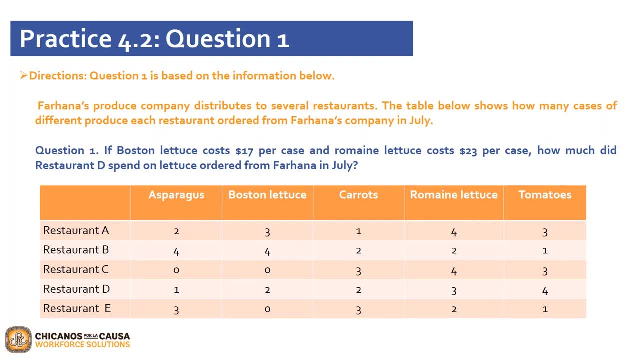 The following says: Farhana's produce company distributes to several restaurants. The table below shows how many cases of different produce each restaurant ordered from Farhana's company in July. Question 1 asks if Boston lettuce costs $17 per case and remaining lettuce costs $23 per. 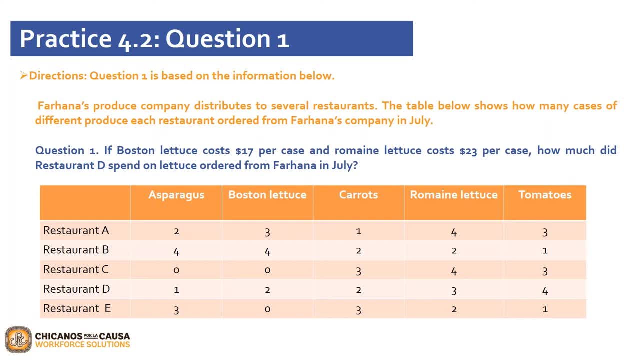 case, how much did restaurant D spend on lettuce ordered from Farhana in July? Would it be A $85,, B $93,, C $103, or D $143?? Please feel free to pause the video to solve and answer this question. 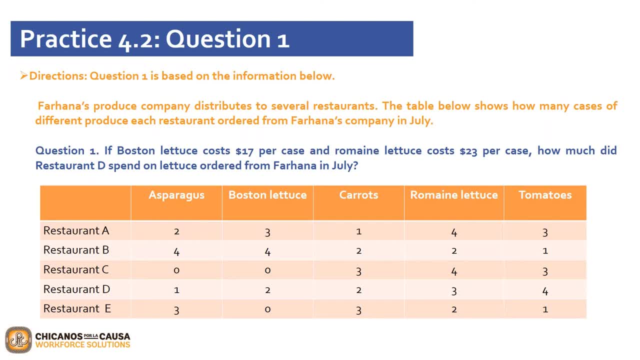 Once you're ready to begin again, please click play. The correct answer for question 1 would be C $103.. Restaurant D ordered two cases of Boston lettuce and three cases of remaining lettuce in July, So you would solve this by doing 2 times $17 plus $103.. 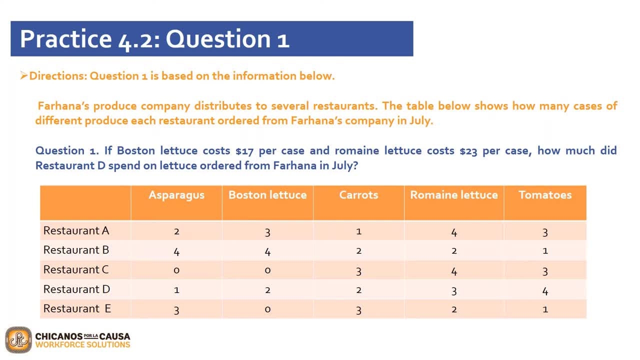 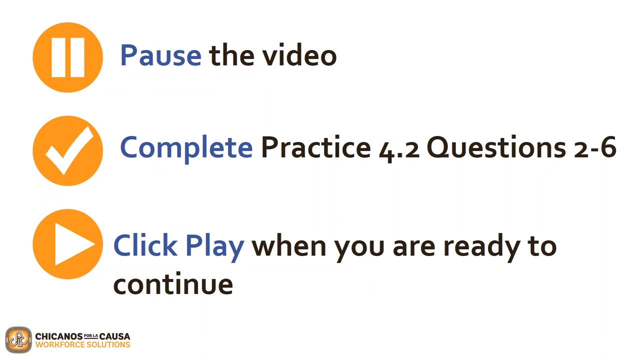 3 times $23,, which equals to $103.. You may now pause the video and complete questions 2 through 6.. Click play when you're ready to continue. We have now reached our final lesson. Lesson 5, Distance and Cost. 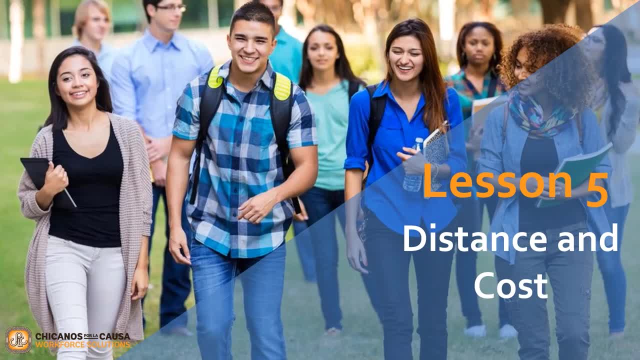 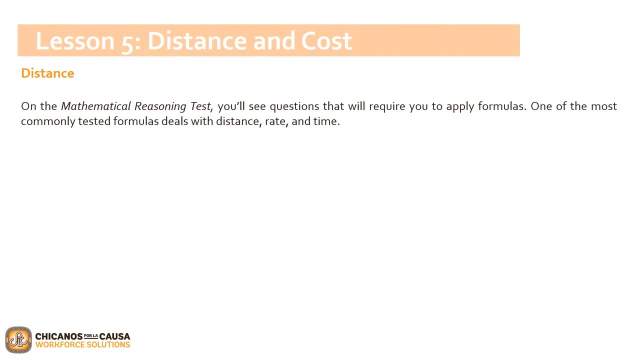 On the Mathematical Reasoning Test, you'll see questions that will require you to apply formulas. One of the most commonly tested formulas deals with distance rate and time. Distance is a product of the rate at which something travels and the amount of travel. 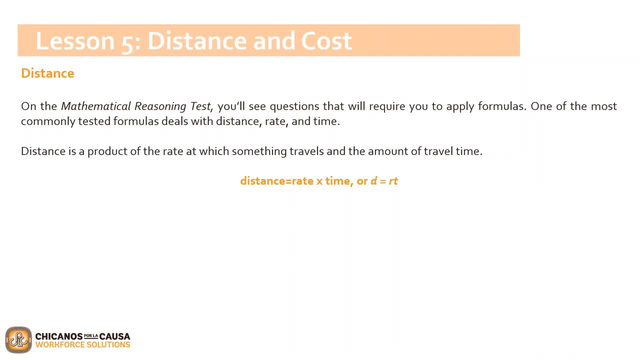 time. Distance equals rate times time, or D equals RT. Distance equals rate times time, or D equals RT. Distance equals rate times time, or D equals RT. Notice that letters or variables can be used to represent the different parts of a formula. 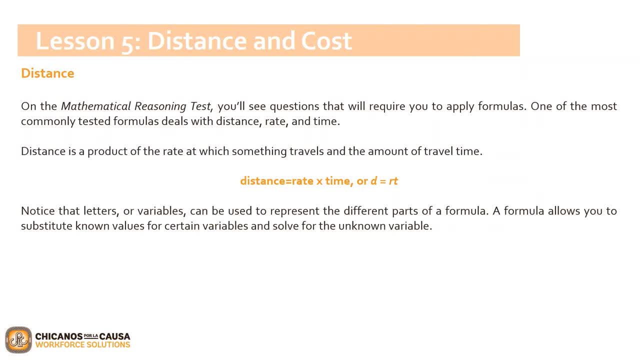 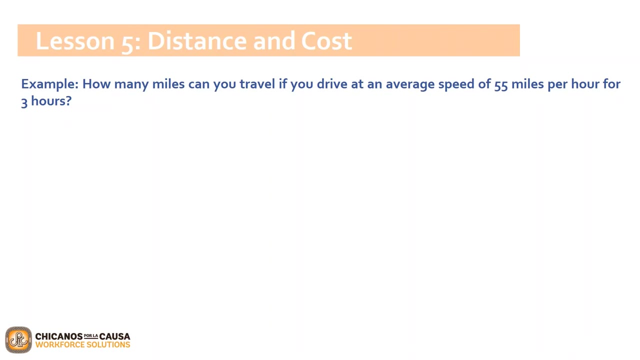 A formula allows you to substitute known values for certain variables and solve for the unknown variable. Let's now view the following distance example. The distance example says How many miles can you travel if you drive an hour speed of 55 miles per hour for 3 hours. 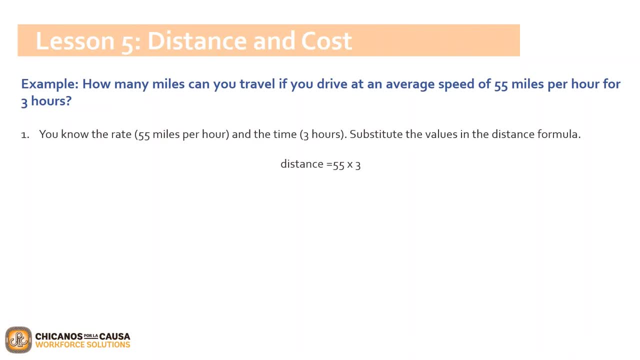 First, you know the rate- 55 miles per hour- and the time, 3 hours. Substitute the values in the distance formula. Using the distance formula, distance equals 55 times 3.. Multiply to find the distance. 55 times 3 equals 165 miles. 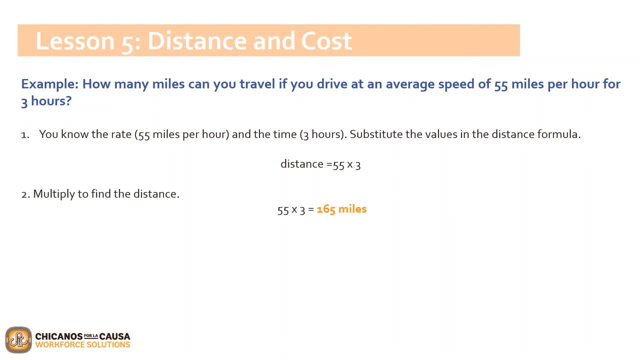 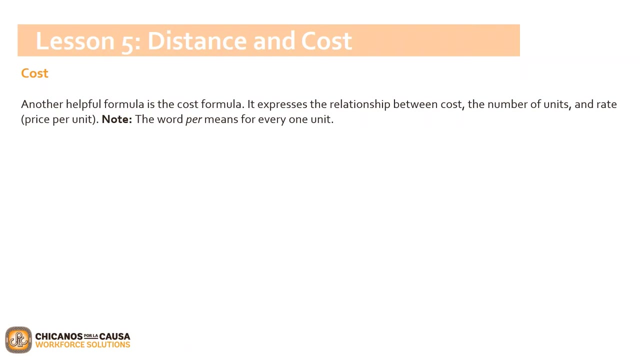 The distance is multiplied by the distance. The distance is the distance, The distance is the distance. Another helpful formula is the cost formula. It expresses the relationship between cost, the number of units, and rate. price per unit, the word per means for every one unit. 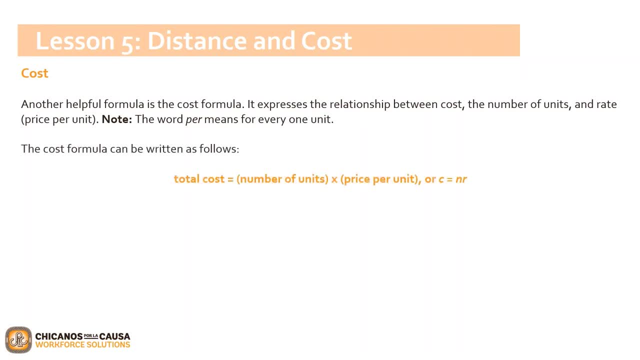 The cost formula can be written as follows: Total cost equals parentheses number of units times parentheses. price per unit or C equals nr. Now let's review the following cost example. The following cost example reads as: at a bakery, a package of frosted cookies is priced: 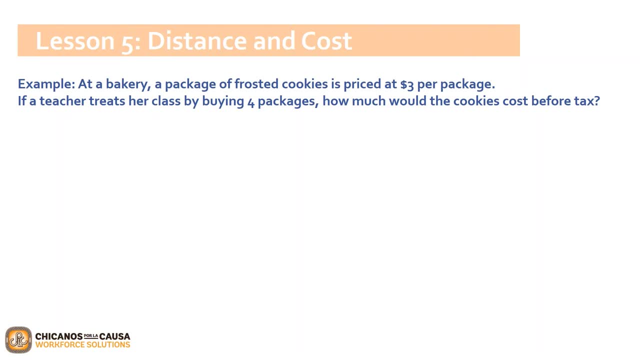 at $3 per package. If a teacher treats her class by buying four packages, how much would the cookies cost First? you know the number of units- four packages- and the price per unit- $3 per package. Substitute the values in the cost formula. 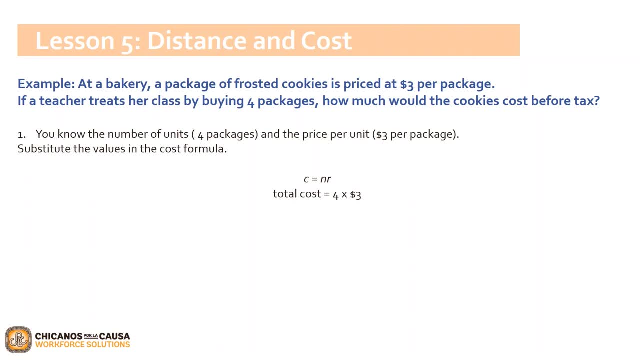 The cost formula is: C equals nr, which would be: total cost equals 4 times $3.. Multiply to find the total cost. So you'd multiply 4 times $3,, which equals $12.. That's how much the cookies would cost before tax. 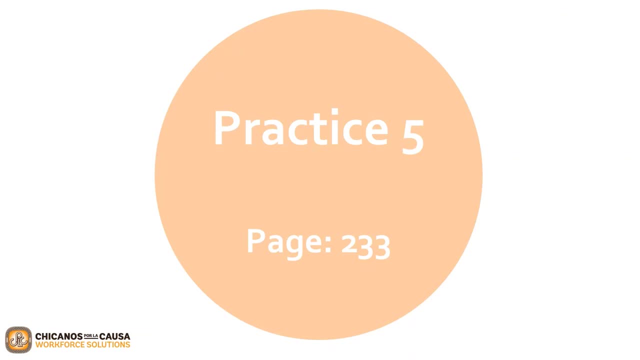 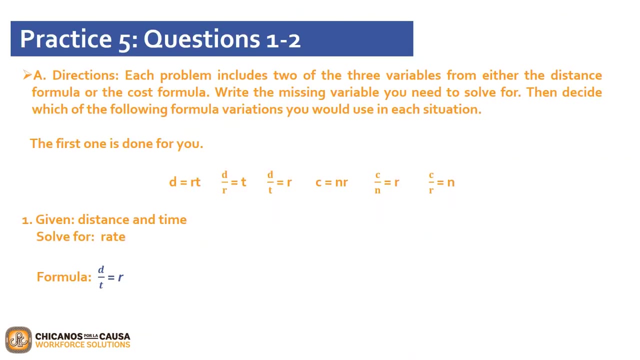 Now that we know more about distance and cost, let's start on practice 5, found on page 233.. For practice 5, questions 1 and 2.. The directions state that each problem includes two of the three variables from either the distance formula or the cost formula. 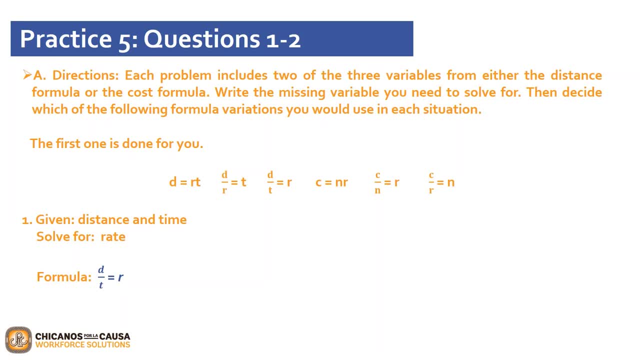 Write the missing variable you need to solve for, Then decide which of the following formula variations you'd use in each situation. The first one is done for you. So in question 1 it says: given distance and time, solve for rate The formula. 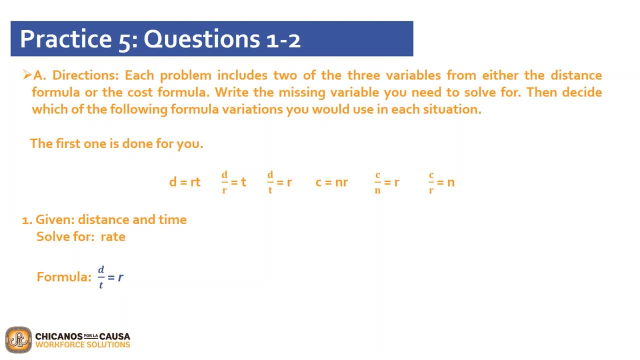 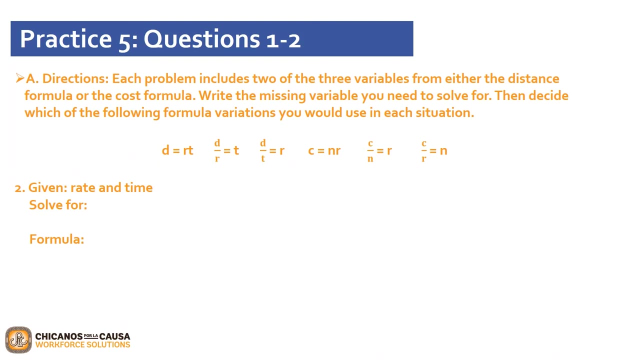 Let's do it again. be written as D: distance over T time equals R rate. Question two says: given rate and time, solve for blank formula. blank. How would you answer this question? For this question you would solve for distance.